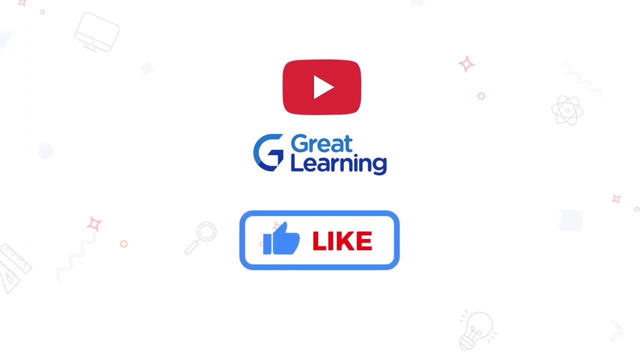 some love and do like this video. knowledge increases by sharing, right. so make sure you share this video with your friends, colleague and everyone who can make use of it. and at the end of the video, if you have any queries or any suggestions and i'll be more than happy to. 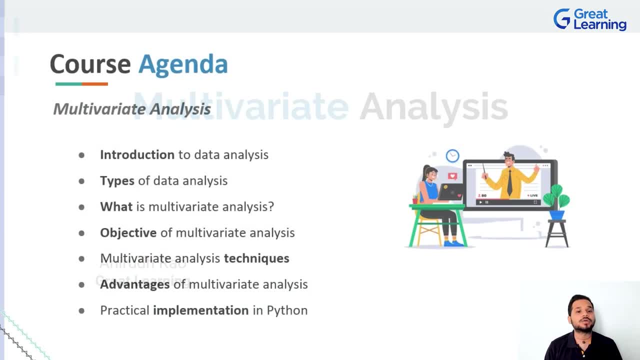 respond to all of your comments. now let's quickly take a look at the agenda for the session. now, when you take a look at the course agenda for multivariate analysis, we are going to be starting out by taking an introduction to understanding what data analysis is in its 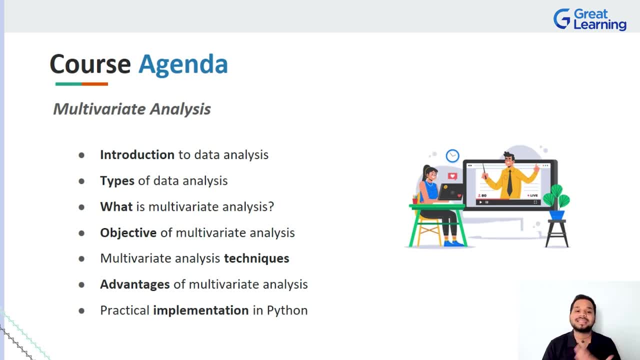 basic terms right, because once you have an understanding of what analysis is, then you'll be very curious to find out what are some of the various types of data analysis that you're going to be using and what are some of the different types of data analysis that you're going to be. 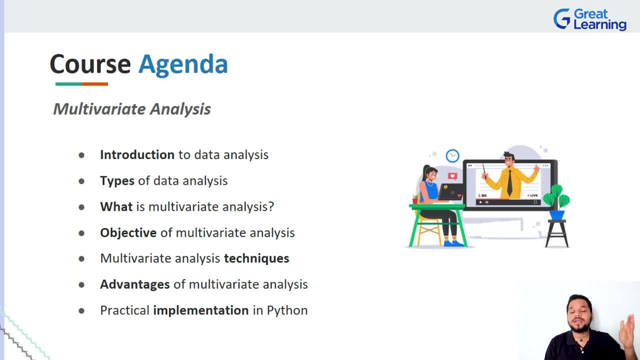 using and what are some of the different types of data analysis that you're going to be using that we have out there? i mean these types. we are going to be dividing it down to the most simplest level. we're going to be assessing, we're going to be analyzing a lot of different things. 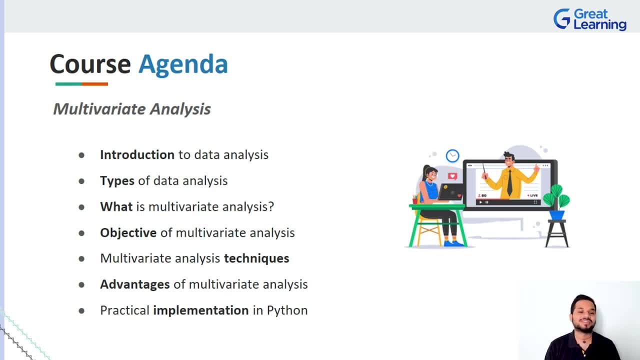 with respect to the various types of it, and as soon as we finish the types of data analysis, the right next thing that we're going to do is we're going to be jumping into the heart of the topic, wherein we will start out by understanding what multivariate analysis actually is right. 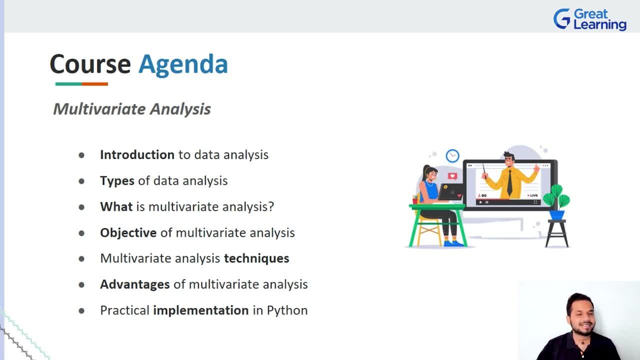 now, once you have a picture of what it is, once you have slight clarity, knowing, oh okay, so this is what multivariate analysis is, you will be very curious to understand. fine, i know what it is now, but why do we use it? what is the primary objective of using multivariate analysis? right, so we're going to take 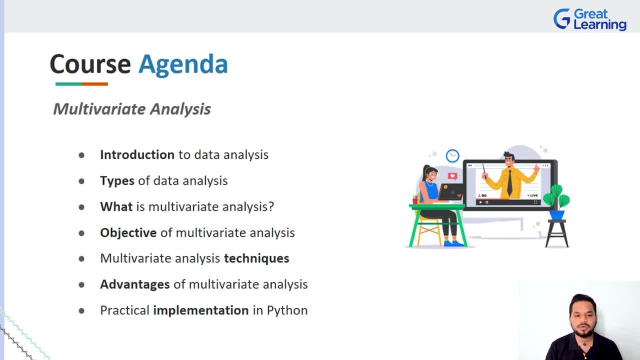 a look at all of that and once you understand what it is, where it is used and all of that, you'll be very curious to say, hey, okay, now what are some of the various techniques that i can go on to use, now that i know the objective and what? uh, multivariate analysis is right, so, of course, 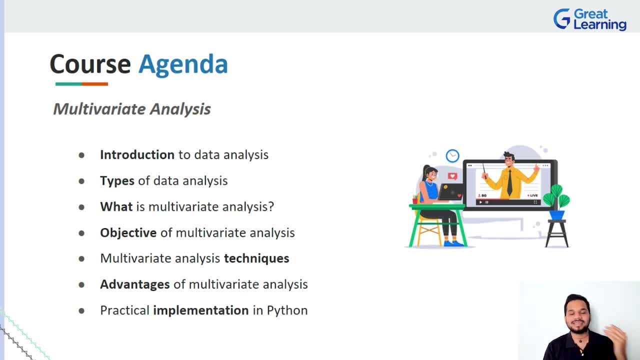 we're gonna have to take a look at the uh techniques as well, and once you understand the techniques and everything there is to know about uh, you know having a good introduction to multivariate analysis- you will be a person who'll say: okay, so what are some of these advantages of multivariate analysis that gives it an edge over. 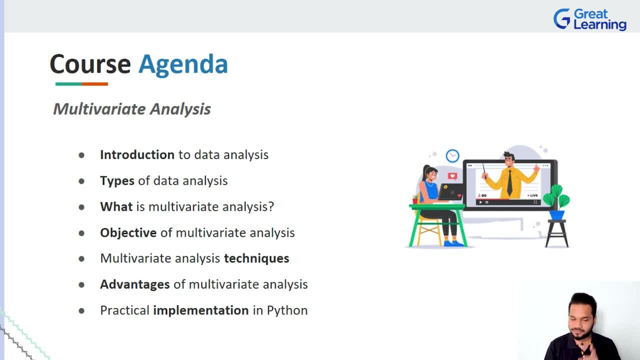 the other types of analysis. right, we're gonna have to take a look at that, and of course we will. and lastly, as you can see, practical implementation in python. as always, guys, anything with respect to data analysis, anything with respect to- uh, you know- performing any sort of analysis. right, it will. 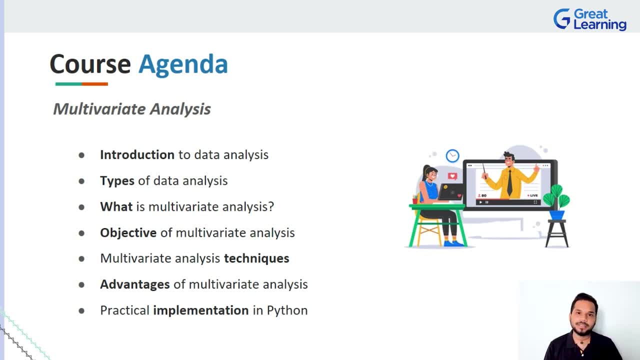 always help you if you always take a practical example to you. know, go and learn, and you will always be able to take the same steps. and then to go along with your theoretical learning and to make sure that, at the end of the day, you are applying whatever it is, uh, that you 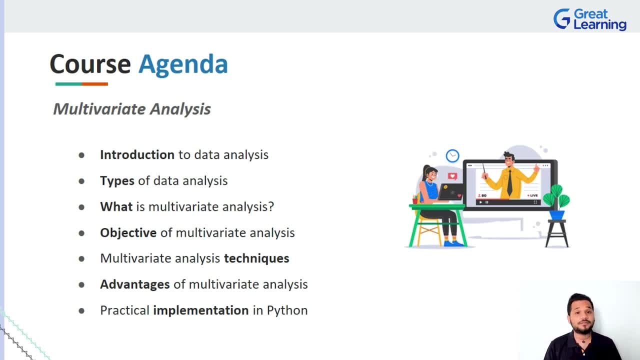 guys are studying and reading and understanding, right. that way, it will help you retain it better and, with the help of a demo, you will understand exactly what it is to actually go on to perform multivariate analysis, right. so i hope all of you all are excited as me, uh, for this course. let's get. 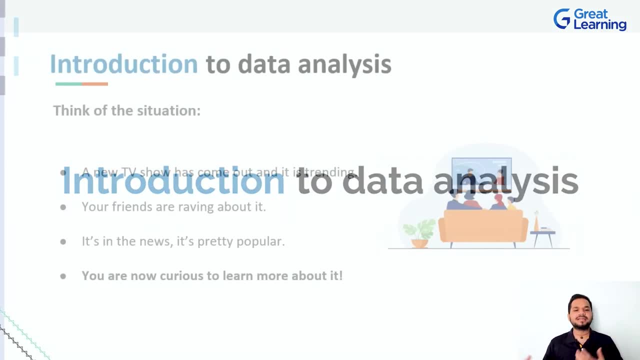 started with the first item on the agenda, which is introduction to data analysis. now, ladies, and is something which is fantastic, because you might not know it's called data analysis, but i can guarantee you one thing: you have used it in your life a lot of different times with things which 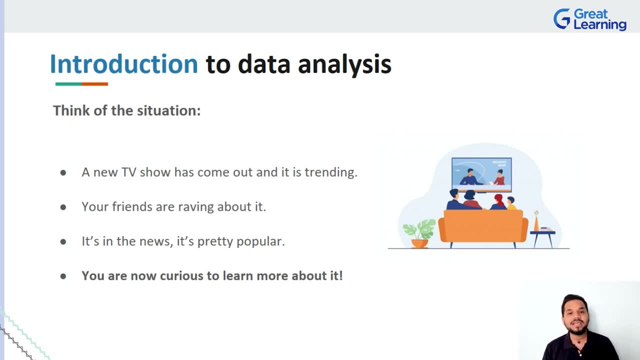 you might have never thought you would have used data analysis, for let me give you a good example here now. think about a situation where there is a new tv show that is coming, or let's just say, season five or season six of some tv show is becoming super popular. uh, they dropped a trailer. 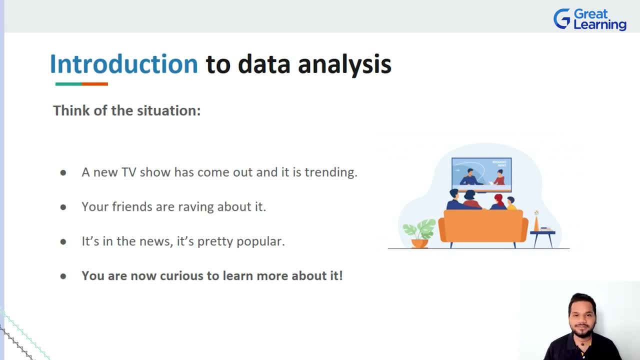 or a teaser or something. the entire world as you know it, now that everyone's connected via social media, everyone will be talking about it. people will be going bonkers about it right when you think about it. so, uh, what do you do when you see a new tv show which says people are saying, oh, this. 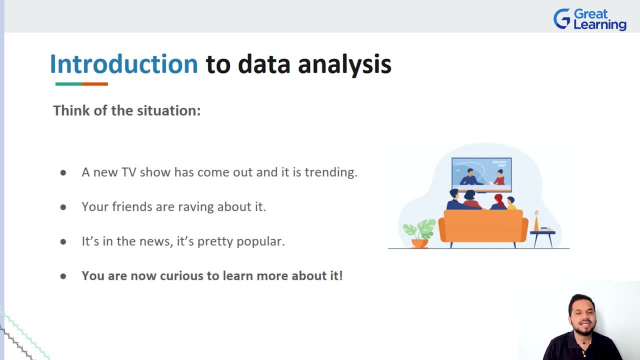 is the best tv show i've ever watched. there is nothing that comes close to this. when people are raving about it and when people are talking highly of it, what do you do? because here is what i do, right, once i figure out something is extremely popular and it is like, uh, you know, growing at a 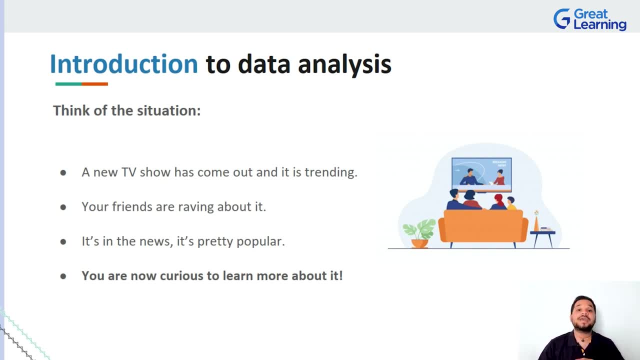 lightning point. i am sure there is something in that show that is making people want to go and check it out, right? so i'm curious now, what i i believe is: hey, okay, so if a lot of people are talking about it, there is something that the show is doing right. so let me find out if, whatever the show is doing, if it. 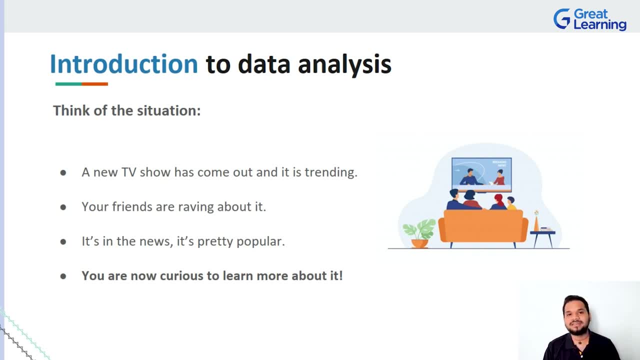 is in my liking or not. now, let's be honest. when it comes to movies and tv shows, we have our own choices. right now, for example, me, i love absolutely what- watching stand-up comedies, or if it's any new tv show or something. i usually prefer comedy or anything on the line. 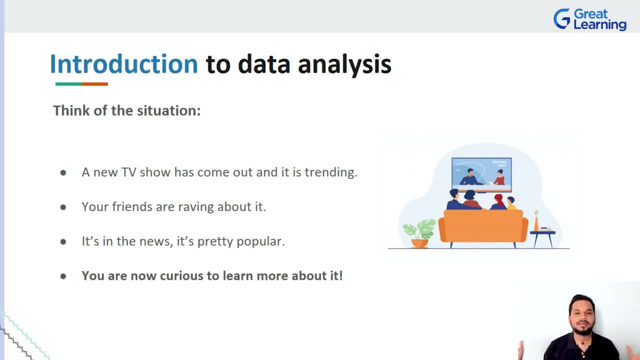 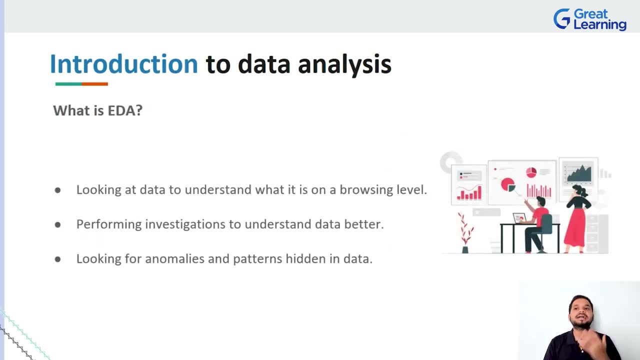 of that. right now, you might be a person who says, hey, i am into thriller and sci-fi tv shows and all of that. so what do you do? you quickly go to google, you read more about it. right, you are trying to understand what it is at its core level. you want to do research, you want to do- uh, you know you want. 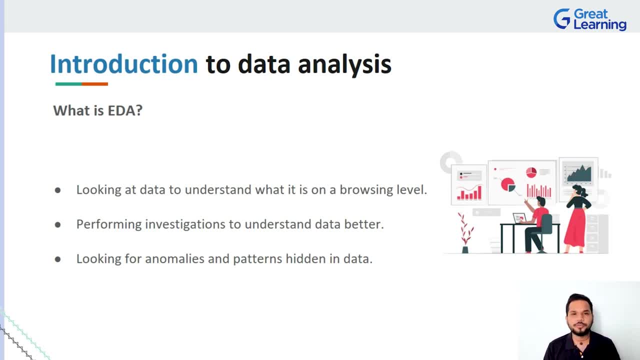 to read some reviews on uh, imdb, rotten tomatoes, all of these review places, to see what people are telling about it. you'll watch the trailer yourself. you'll talk to a couple of friends. now, what is this entire process that you're doing? you're trying to figure out. what is it that you're? 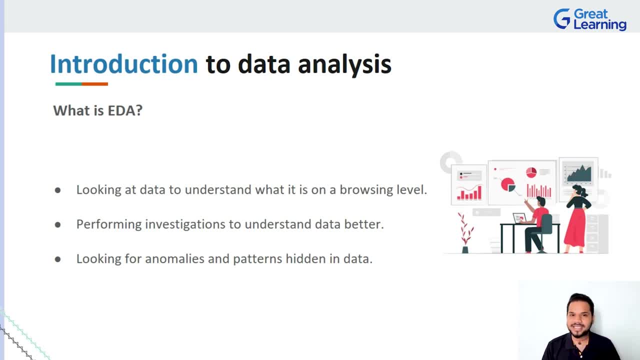 trying to explore more into the topic right now. look at your screen. it says what is eda? eda stands for exploratory data analysis and, ladies and gentlemen, to a good amount of extent you guys were doing exploratory data analysis there because you knew what the problem was. the problem was you. 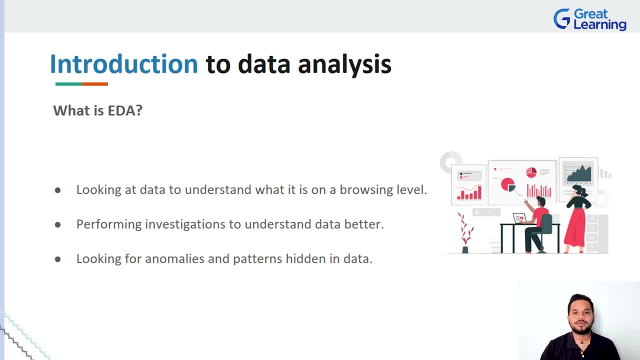 don't have enough information about the tv show. now you know how to solve. it is actually by watching the tv show. but before committing to watching the tv show, you realize saying let me do a little more research, let me do a bit of analysis to see if this tv show is for me or not, and then you can. 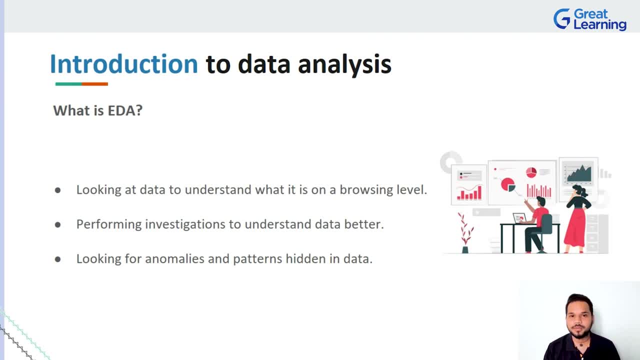 see if this tv show is for me or not, and eventually you did everything that you would do and then probably you either watched it or you didn't watch it right. so, taking a look at understanding this in the data analysis perspective that we're taking a look at right, it's basically you having a problem. 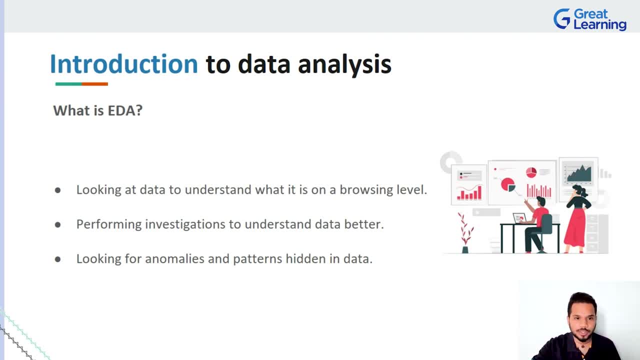 you have certain data and you know that the data can be used to solve the problem. but as it is, if you just look at the data, it will not really give you any sort of insights. it will not give you patterns just by looking at it. right, you have to perform some investigations on it, you have to work. 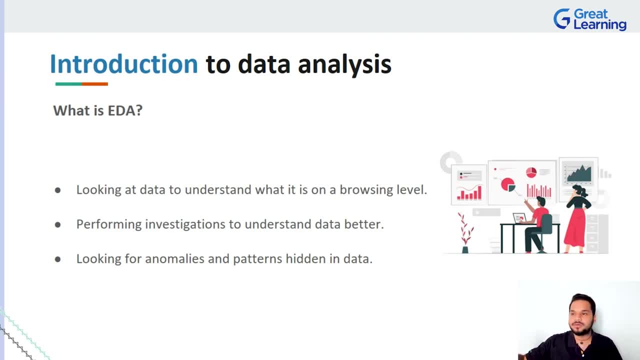 on it deeper now. if i give you a single brick up, you know a couple of bags of sand and a bag of cement and tell you, hey, build a house. right, if i just say, build a house, do you think the house is going to be built? not really. you're going to need people, you're going to need some process further. 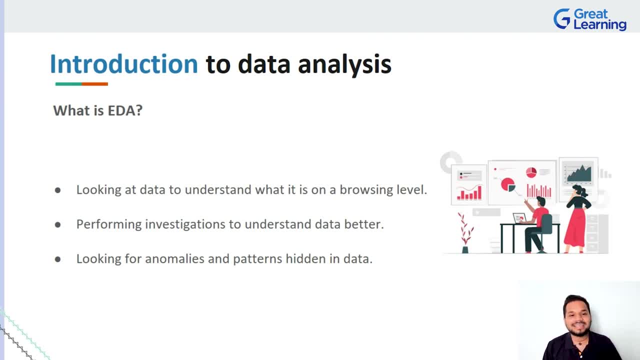 to actually use all the raw materials to build this data analysis. is that raw material where you're actually investigating, right? that is very important for you all to understand now. there are so many things that is hidden in data that you will not realize as soon as you look at it with. 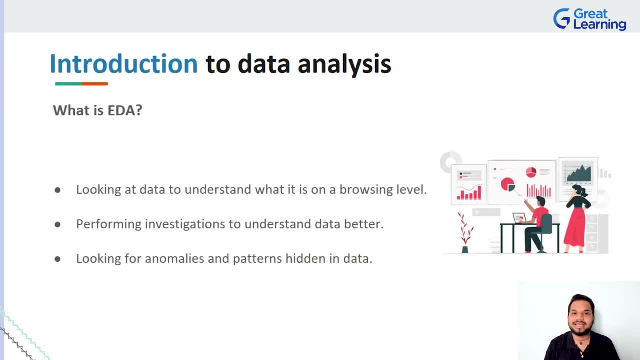 your eye. you can look at data with your eye and say, okay, well, there's not really anything that i can tell. there's a lot of rows, a lot of columns and you know we have certain data and you can probably guess what might be happening. guess, right now, i can guess that it will rain tomorrow here in. 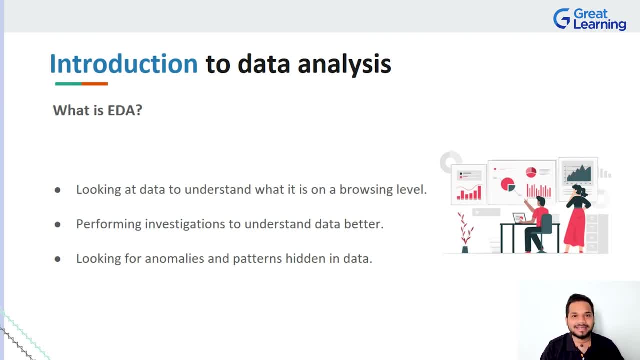 bengaluru. but what? how sure am i? i'm just guessing, i'm just seeing it. it doesn't mean it has to happen. but that is where data analysis is very different. here, when you make outcomes, when you predict something based on your data, when you're analyzing data and you say: here is the result of 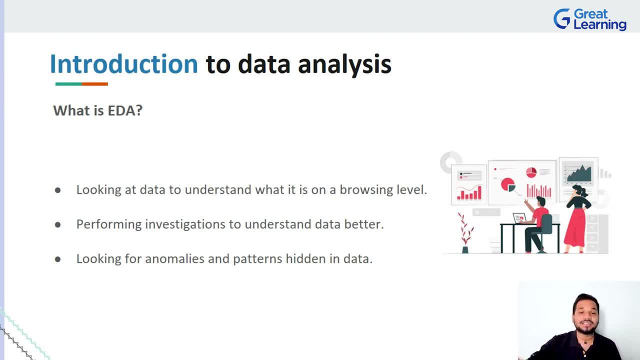 the data analysis. basically, what you're saying is: hey, i know that this might happen tomorrow. here is the data to prove that it will happen tomorrow, right now. there, you're not guessing anymore. you have data ready at your hand to back everything that you have to say right now. if i say hey, 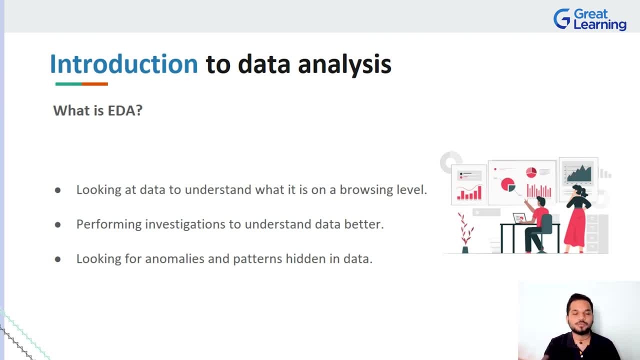 tomorrow it's going to rain because this is the precipitation factor. these are the clouds. that's how it's moving around india. you can expect a ton of clouds to be on bangalore tomorrow and there's a very good chance it might rain. now, when i say it this way, you'll be like: oh okay, it might rain. 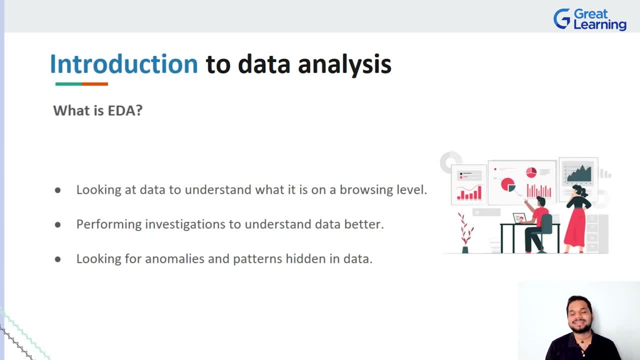 correct rain now. think about it now. this exact small example that i gave you. uh, you know, this kind of an approach to understanding data is what is making it a key part of millions and billions and trillions of dollars worth of businesses today. right, everyone around you? i bet everyone right. 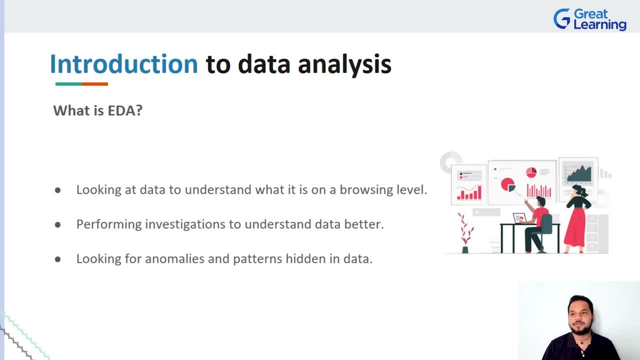 from the grocery stores near you all the way to someone- uh, you know, in a very big company, maybe like google, facebook or something. these guys are using data analysis on a day-to-day basis. of course, not everyone is sitting and working with algorithms, creating models and all of that. 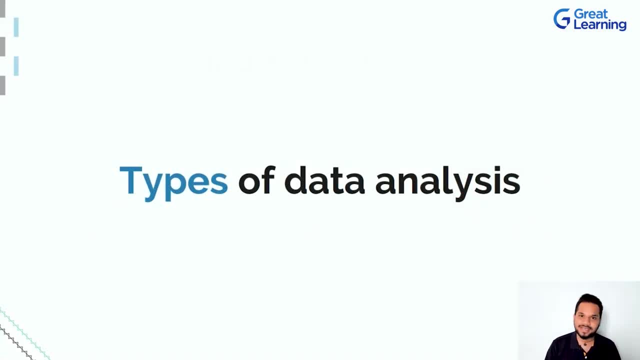 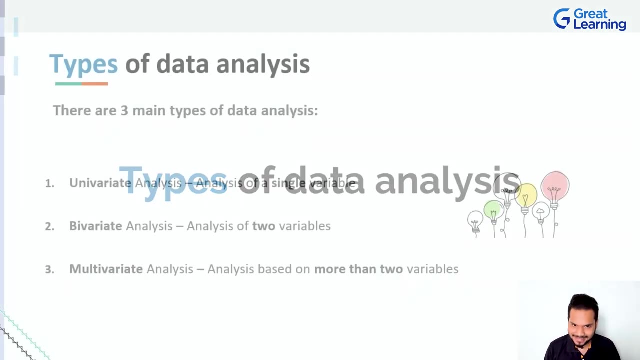 but they are, in their own way, performing some sort of analysis right now. you, you closely observed what i just said: some sort of analysis. so what are the various- uh, you know- types of analysis that one can go on to perform? uh, you know when we're discussing about data analysis right now, ladies, 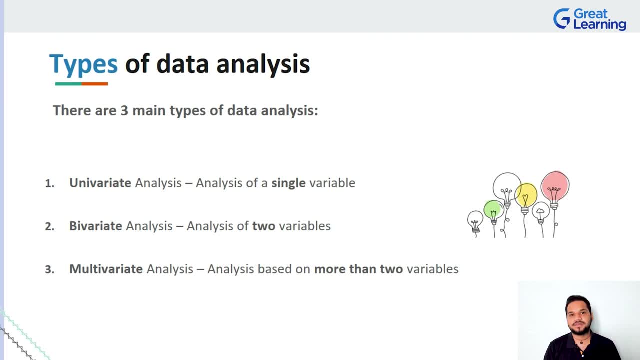 and gentlemen, you have to understand that there are three very important types of data analysis out there. it is not just multivariate analysis, we have univariate analysis, we have bivariate analysis and we have multivariate analysis as well. now, with respect to univariate analysis, it is very simple: what does uni stand? 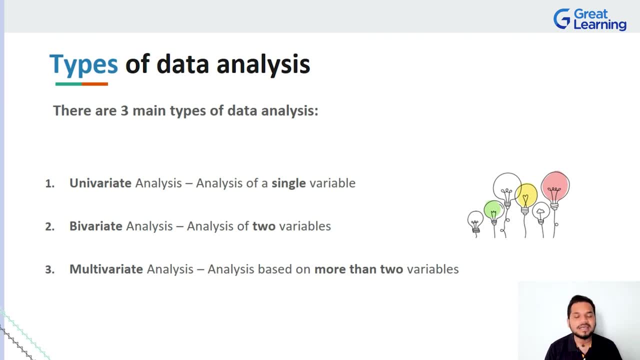 for all right. uni stands for one, uni stands for single. so, whenever you are assessing and analyzing a single variable which will have an impact on the outcome, that is when you you. that is when we use univariate analysis. now, when you have to analyze two variables which will tell you which, 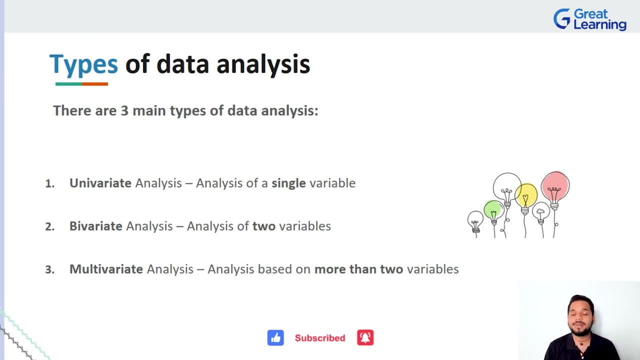 will have an effect, it will have a say on the outcome. that is when you use bivariate analysis: one variable done, two variable done. what if there is a case where we have more than two variables that we will have to analyze and assess again. you figured it out by now, right, it's multivariate. 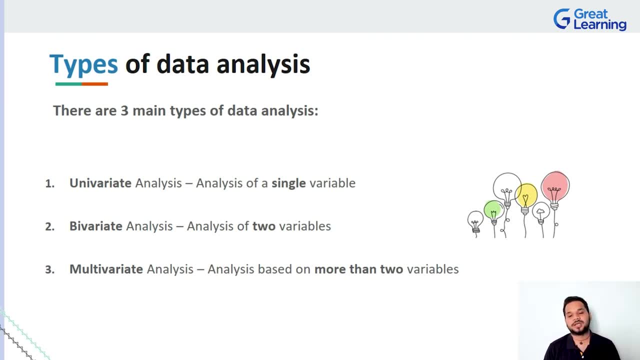 analysis, which is basically used whenever you have to work with two or more variables. now, ladies and gentlemen, do pause for a second here and try to understand and see if you can find any example cases of where you might have used univariate analysis, bivariate analysis and 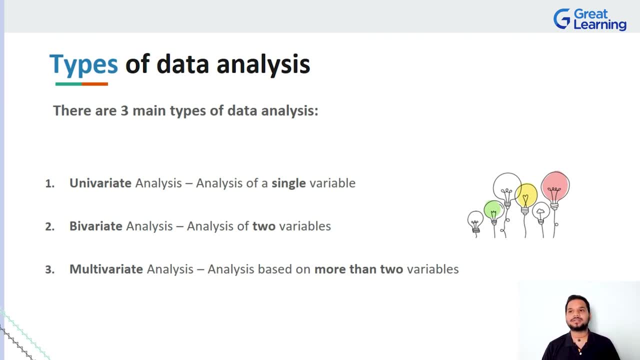 multivariate analysis. right. if you're just analyzing one thing to see if it is right or wrong, that's univariate. now, if you have two objects or something that you'll have to assess to see towards a common outcome, that is bivariate analysis. now multivariate analysis. again, there's a. 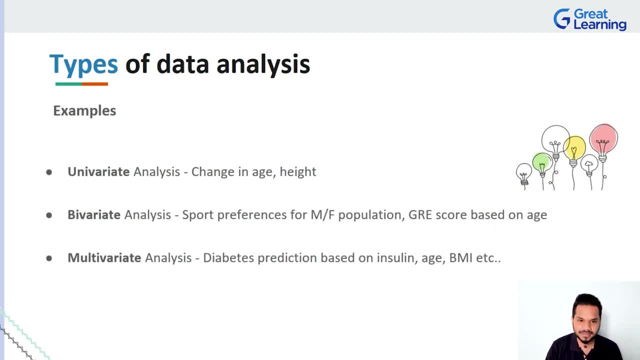 lot of factors that are involved. right, in fact. let us discuss these examples. univariate analysis: when someone says, hey, analyze the change in the height of a particular person in majority of the cases, how do you think it goes right? so when they're young, the height is pretty much very. less and as they go in age- the age of 18, 20, 25, 26- they reach certain age and they tend to plateau at that age for a really long time. so it's a linear growth right. it's not like one person grew 10 feet. 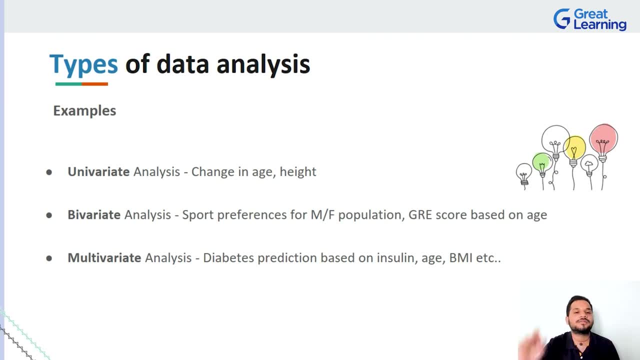 in a day that really doesn't happen. so it's only one variable that you have to assess. to give someone the height, right, you just have to assess, measure them and tell them: hey, this is one of the variables, this is one of the uh, uh, you know. 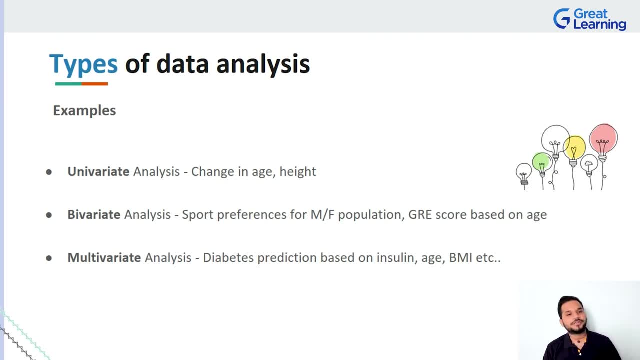 important things that will help you get to the outcome. simple now, if i say hey, analyze the change in someone's age. right, age is still a single factor, right, you don't have to consider anything else apart from, uh, if you know the person's age, that is all is, let's just say, required for the 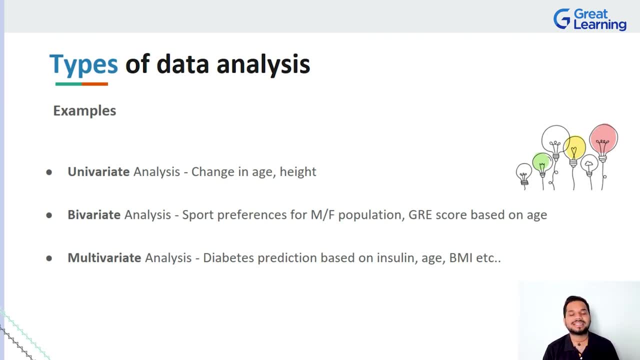 analysis result. multivariate analysis says that if you only want to assess and analyze age, or not just age, this is an example. uh, this is what will lead to having one variable deriving and helping you get towards your outcome. this is univariate analysis. now take a look at bivariate analysis. right, bivariate analysis is fantastic because here you will be. 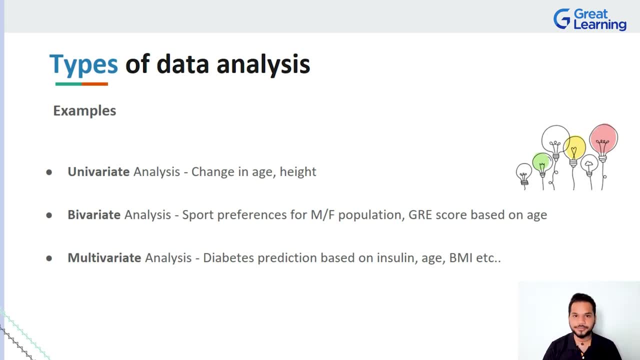 taking a look at understanding two parameters at a time. let me tell you, uh, so think about sport preferences in our country, right? so, uh, not just in our country, it's just a hypothetical example out here. uh, whenever you're thinking about sport preferences, it is very common that you know, guys. 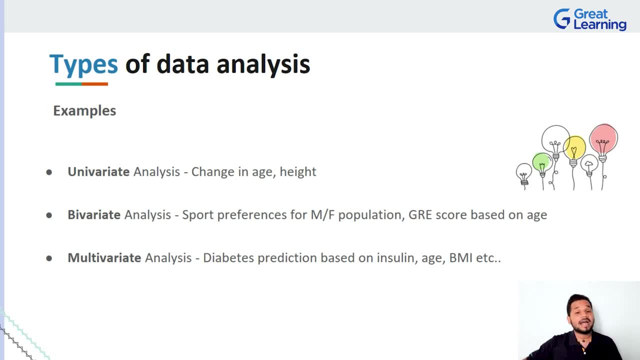 would love to play football on the national and the international leagues, and women see themselves, uh, you know, mostly in archery. uh, when you take a look at all these track and field events, which are again extremely difficult in my opinion, right, so if you say, hey, what are the sport preferences? 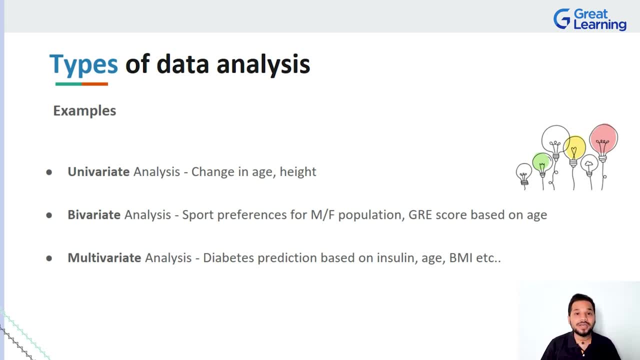 for male population and female population. look at this. you have two uh things that you'll have to assess and out. you have to assess your outcome based on right. so male population: they will have their own choices. they will have their own uh sport that they like. now, if someone asks you a question, saying, hey, at that point of time in 2005, what were the? 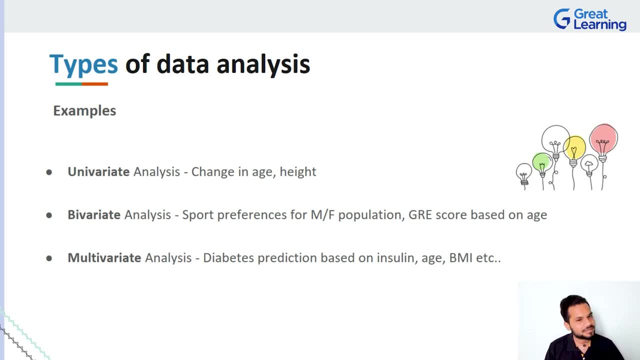 uh details of uh. you know the male population. what games were they playing? can't you answer that? yes, you can. if the same question was asked in the case of female population again, you would have analyzed a lot of different sports to get to the conclusion to say, hey, females in the year 2006. 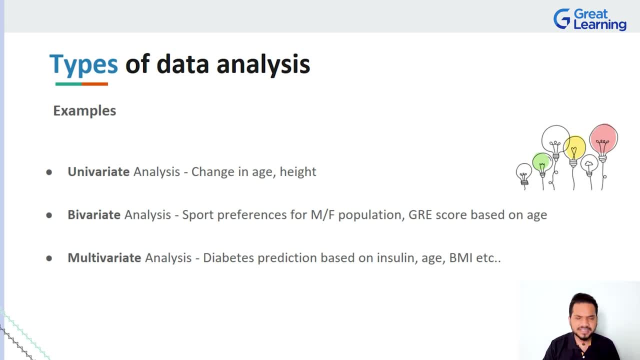 were playing these mini games. simple, right, so you can do it. another example for bivariate analysis is the gre score based on your ages. now, when someone tells you that you know you're playing you, hey, i want you to take all the gre scores of all the students who have written the exam. 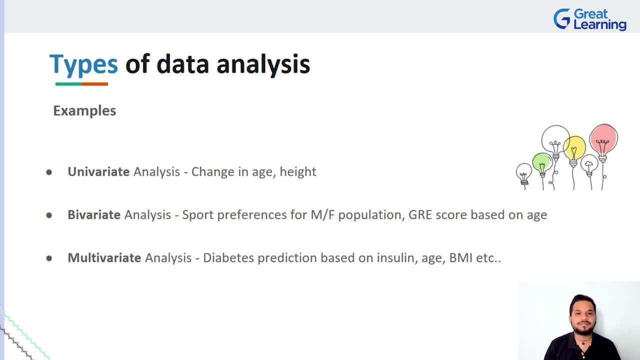 uh, divided based on their age. now you have two things that you'll have to filter something based on. first of all, you have to pick up all the gre scores. next, you have to pick up all the age of the those particular candidates who have written that examination and eventually, then you can perform. 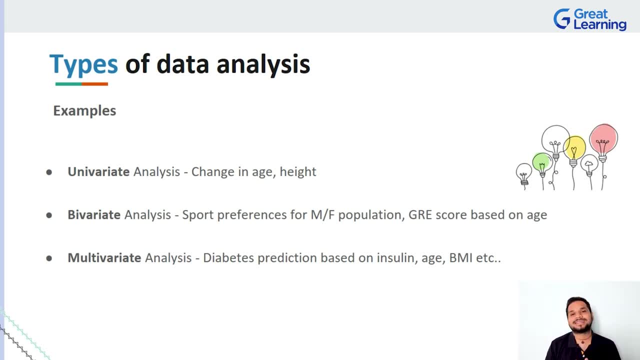 some analysis. there are two inputs, there are two variables. you're assessing here the score and the age at the same time, right? so this is bivariate analysis when you take a look at the score and the age at the same time. right? so this is bivariate analysis. you have got the game. 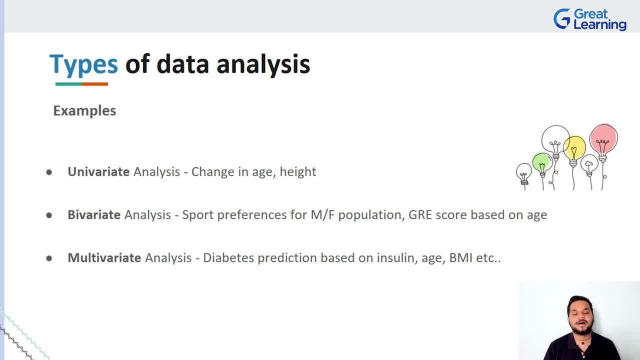 by now. right, so you will have to have more than two variables to actually check if a person, uh, you know, to check if an outcome is being achieved there or not. in the example that you can see here, it says diabetes prediction using insulin, uh, age, bfi, etc. right, in fact, we are going to take a look. 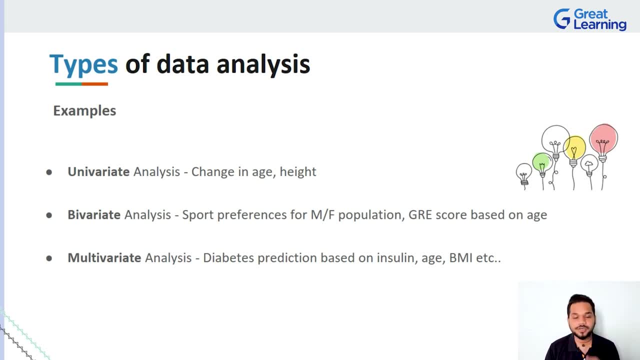 at a practical demonstration on the same particular topic. uh, it's an absolutely fantastic demo because here, just think about the real life diabetes, uh situation, right. uh, there is never only a one reason that will lead to diabetes. right, there's many factors, there's age, there's genetics. 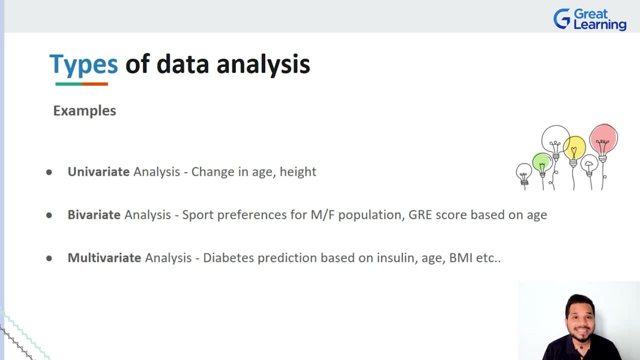 there's insulin. there's your diet, which matters a lot. there's your exercise habits- uh, you know your blood pressure. there's a million things. there are so many variables and if those variables fall into place, there's a very good chance that you might have diabetes, right? so this is again. 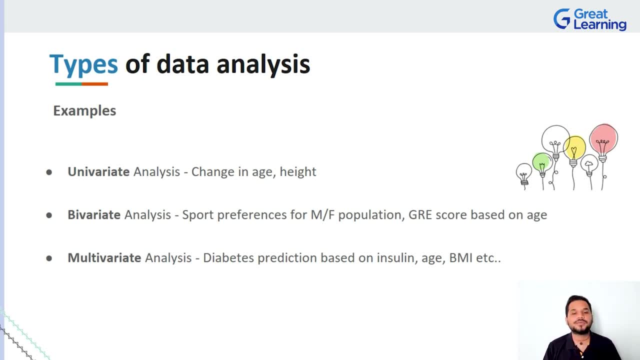 a common problem in today's world and we are going to be using the power of machine learning to actually assess and analyze and perform multivariate analysis on it, because, at the end of the day, we will know that, hey, diabetes does not just depend on one factor. 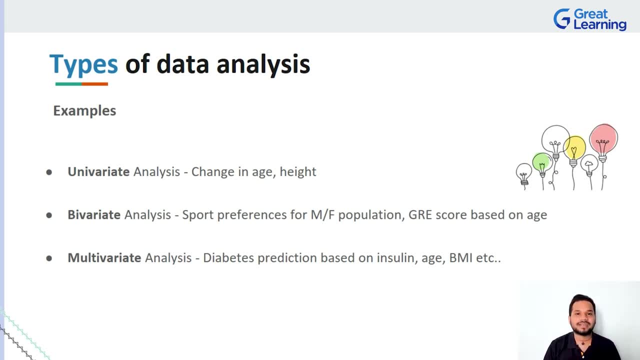 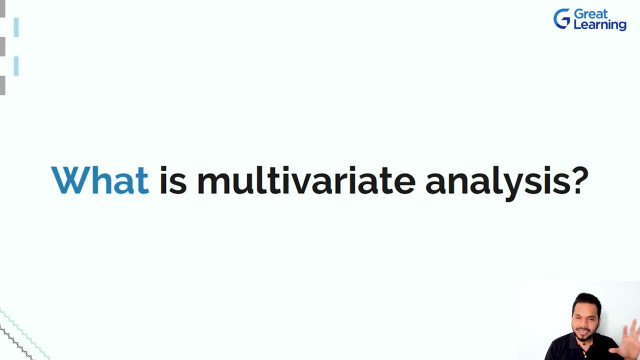 it depends on multiple factors, so let's have each of those factors, let's perform some analysis on them, right? so, guys, these are the various types of data analysis that we have out there. now, coming to the heart of the topic, what is multivariate analysis? right, we took a look at examples. we 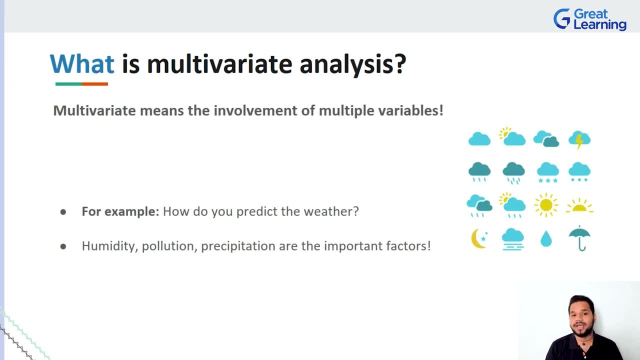 understand that we're gonna have to have more than uh two variables to work on it, right, uh again, i can give you one example, some multivariate analysis, because, as i told you, multivariate analysis- unless you search for it in your real world, you would not know you've used it. think about it, right. multivariate thinks about. 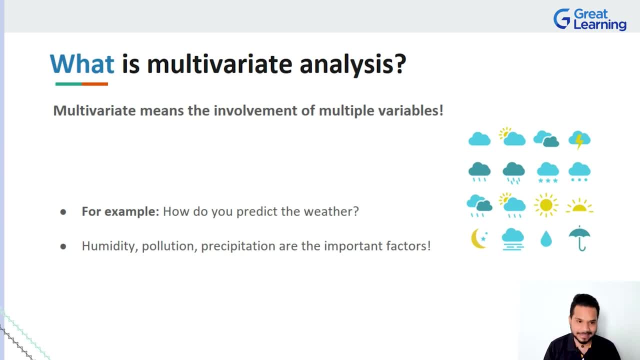 talks about always making use of multiple variables at a time. the same weather prediction example. i spoke to you at the start. if i'm just telling you tomorrow it's gonna rain, it's an absolute guess. right, it can be the sunniest day in the country tomorrow. but what if i tell you, hey. 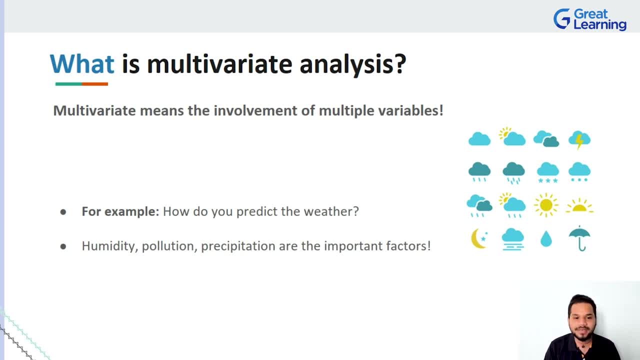 tomorrow it's going to rain, because i assessed these many, these many parameters. for example, a rain might depend on humidity, it might depend on pollution, it might depend on precipitation, it might depend on a ton of different other factors- right, all these numerical factors or categorical factors that will lead to that outcome of it raining. uh, tomorrow, now, when that is the case, 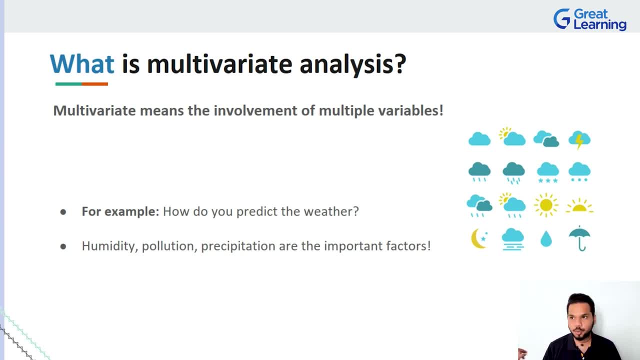 you have to be- uh, you have to understand for a fact that it's not just one thing that lead to it. there's multiple things, and weather prediction is actually a very good example, uh, for all of you all, to actually understand multivariate analysis. right now, let's see how it works. 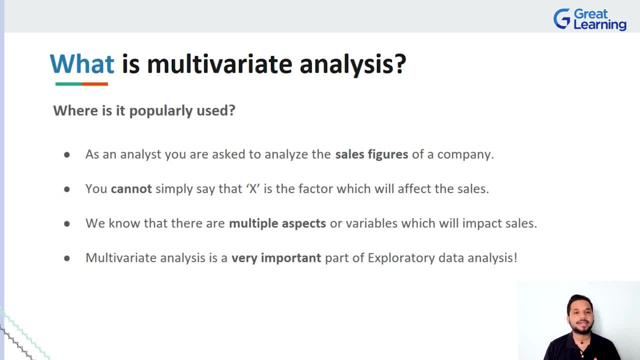 uh, you might be a person who might be saying at this moment of time: okay, i know, uh, what multivariate analysis is, but where is it popularly used? well, we're going to be discussing a section just for that, but let me quickly give you some key pointers out here right now. whenever you go to an analyst, 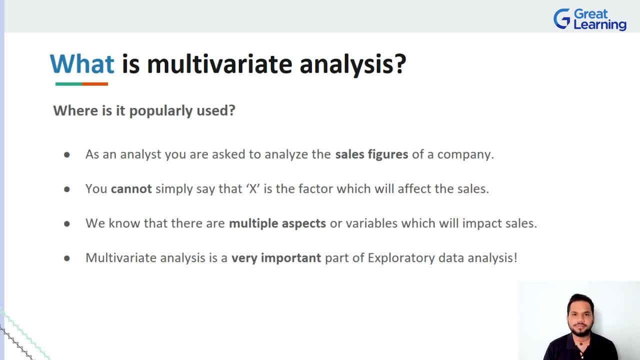 and say: hey, what are the sales figure of my company? now, you might be a person who might have just opened a brand new chocolate uh company. you're selling chocolates, right? uh, you will know that during this time- september, october, november, december- uh, this is when people usually 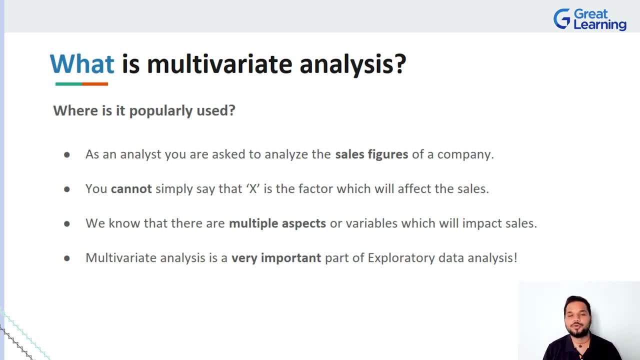 tend to sell a lot of chocolates, right? because again, it's christmas time, it's new year time, there's halloween. there's always something coming around, uh, these particular days. so you might be, uh, you might be, a person saying, hey, i want to use the last six month data that i have to try to see if i 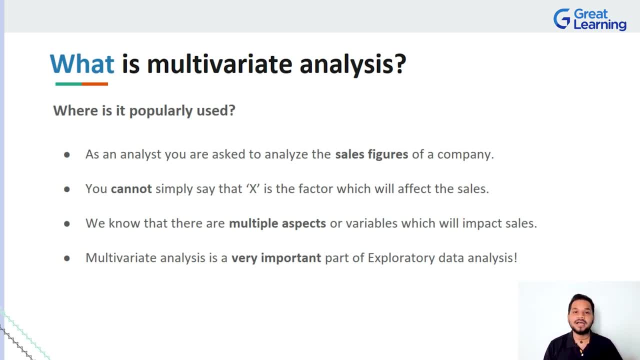 can predict what my sales will be during christmas. or, even better, i'm going to give you the data from last year's christmas sales and can you guess how many customers that i can expect this year, so that i can order so many chocolates for the customers, right? so when you think about it, you can. 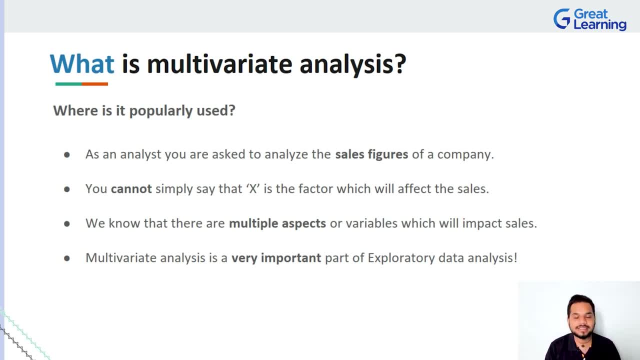 sort of questions where probably 20 years back, you could never answer those right. and now you can not only just guess out, guess it out or something like that, you can have data to prove everything that you're saying. now it is very easy to say: hey, you know, get 10 chocolates. how do you know it's 10? 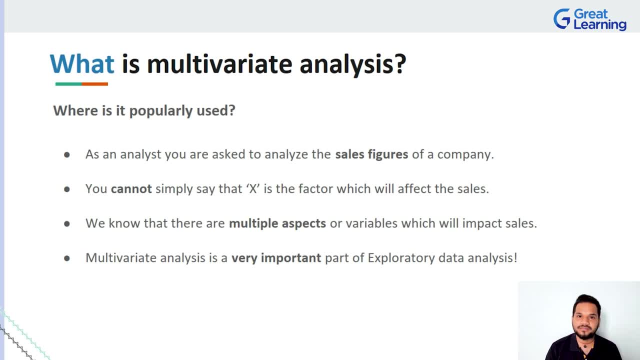 chocolates. right, you cannot just say this is the factor which might be affecting the sales of any particular company out there. there's multiple aspects, there's multiple variables, there are so many dependencies, uh, which will lead to a situation such as this. right, so you're going to have multiple variables and you're going to have multiple analysis. so it is very, very important. 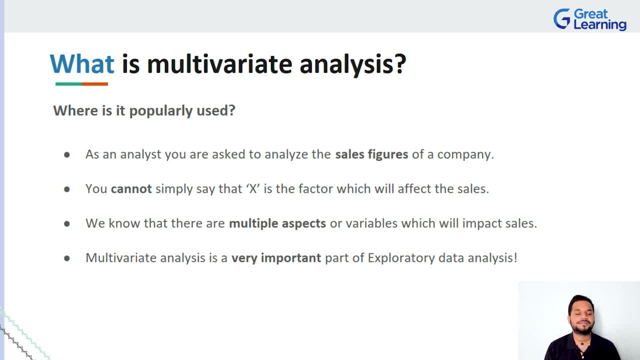 multivariate analysis- you have to understand, ladies and gentlemen, is a very important part of uh, this domain that we call as exploratory data analysis or eda. so the next time, whenever speaks about eda, understand that multivariate analysis is a very important, has a very important role. 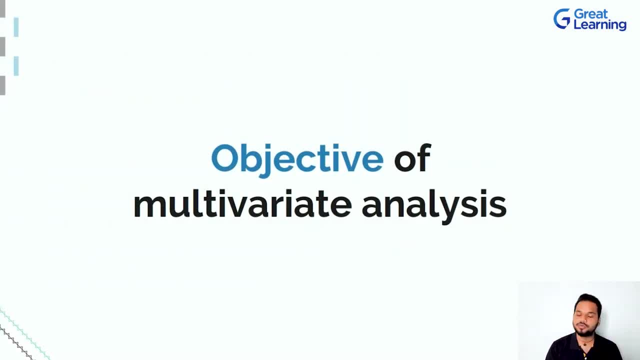 uh, to play in that right now. once you understand where it is popularly used, you will be very curious to take a look at knowing, uh, the objective of multivariate analysis. we saw what it is, we saw where it is used, we saw, to a certain degree, how it can be used, and all of that. 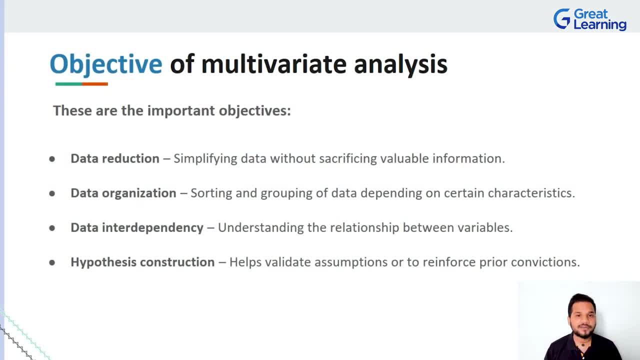 as well. but what is the overall objective? why are we doing multivariate analysis? now, ladies and gentlemen, multivariate analysis is basically done because of the following objectives. you see on your screen right now, the first uh point says data reduction. now, whenever you are performing analysis, whenever you're using multiple variables to analyze something, you can actually come to a point. 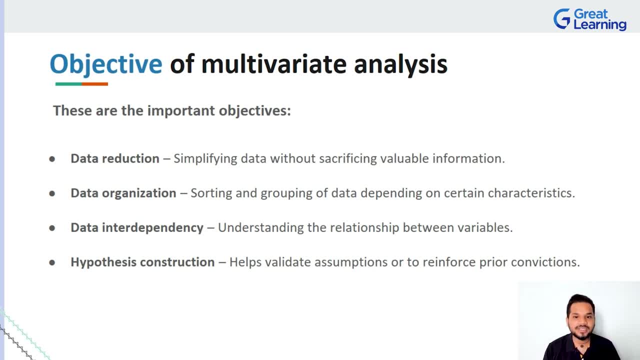 reduce your initial data because you might have had it in better categories, or you might be simplifying a very, very complex data set into something really simple and at the end of the day, you're doing that. here's the advantage: you're doing that without having to sacrifice any valuable. 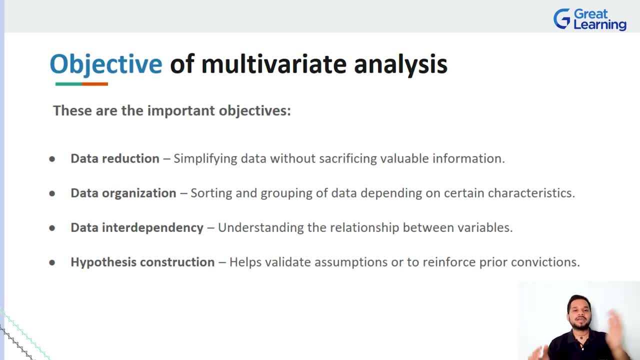 information. now, if i tell you, hey, here is this large chunk of data, here is this, here's the same chunk of data, but in smaller size, you might be the first person to say, hey, did you remove any data to make it smaller? well, with the case of this type of data reduction, you can. 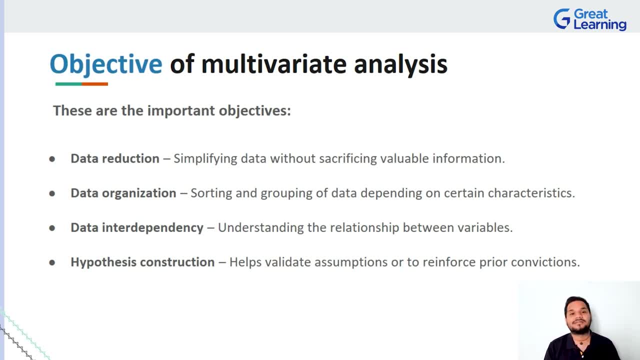 reduce the size of the data without having to sacrifice something which will add meaning to the whatever problem it is that you're trying to solve. this is critical for you guys to understand, right? take a look at the next point. it says data organization now, whenever you're trying to perform. 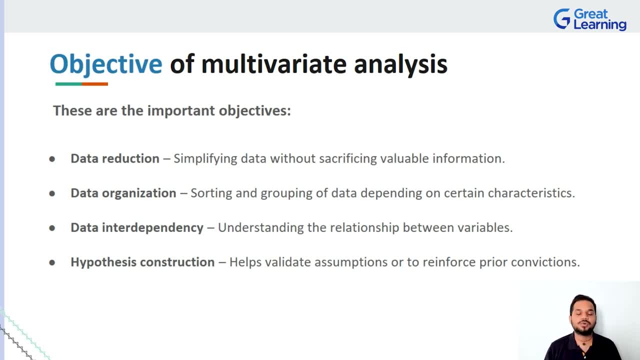 multivariate analysis. it never is the case that, hey look, these two uh parameters are the only reasons why this might happen in in that particular way. no, there might be many cases where you'll actually have to go out to sort your data or group your data based on certain 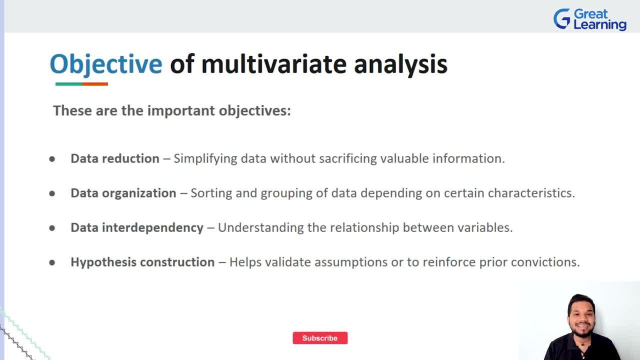 characteristics for you yourself, to get some visibility, to say, hey, okay, now, uh, you know we can go on to. now that i've grouped all this data, i have a clarity of what variable has what effect on the data, and now i can sit and perform multivariate analysis. right, so an objective. 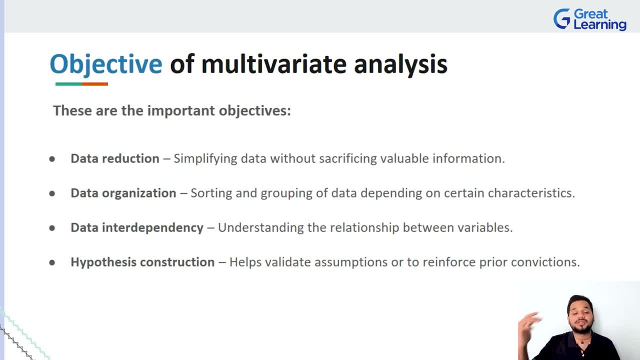 is to actually reduce the data to its simple form. another objective is to actually organize the data, and here is a very, very important one: data interdependency. think about it: if we're talking about multivariate analysis, you're basically trying to understand the various relationships that exists between all these. 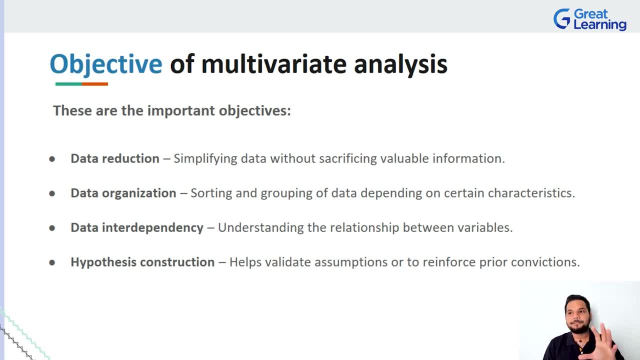 variables that you have out there right now. uh, think about this particular situation: age and fitness. how does it affect diabetes right now? as and when your age progresses- you know, when you're 50 or when you're 55, you might not be able to run like an 18 year old kid, like a 16 year old kid. 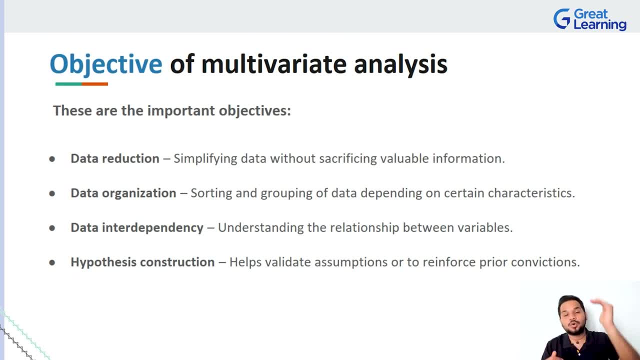 right. so your fitness might come down slightly while your age is going up. now there is a relationship in itself. as you progress in your age, there's a very good chance your uh performance in terms of uh exercises, in terms of fitness, in terms of working out, might slightly come down because, again, uh, in general we say hey, it's an. 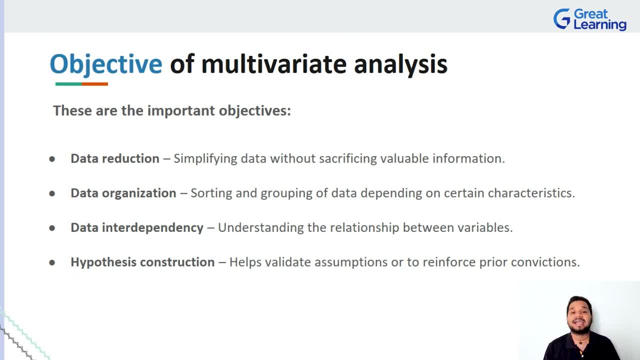 age factor, but it's a direct comparison between age and, uh, you know your level of fitness, and when we see it in conversation, you don't realize that it's again, uh, the interdependency that we're talking about. but now that you understand this, the next time you look at situations like that, 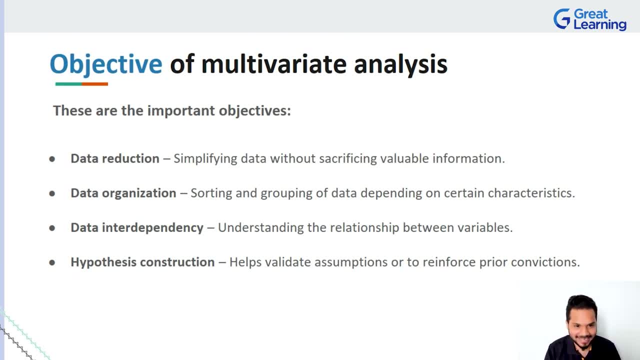 i'm sure you're going to be thinking about data interdependency, right, fantastic. the last point says hypothesis construction. now, ladies and gentlemen, uh, hypothesis constructions are very, very important, because hypothesis is something that you say that, hey, this might be right. right now, uh, you might say that pluto is a planet. there was a time in the world where everyone agreed pluto is a. 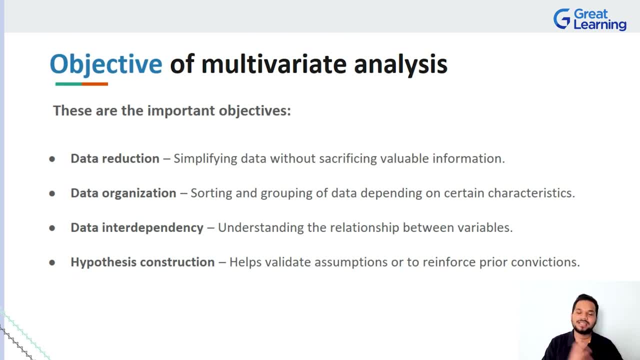 planet and then, i don't know, it all went to bonkers. people don't uh, you know, there's one side of the community that says pluto is still worthy to be a planet. there's another side of the community who says no, pluto is too small, too far, uh, to be a planet. right, so, having a hypothesis, 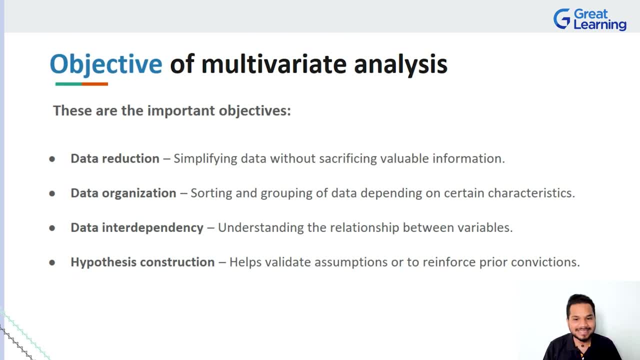 that says, hey, pluto is a planet, going to be a wild guess. it's going to be you actually having to say, hey, pluto is a planet for so and so and so reasons correct. so to give out those reasons, you must perform some analysis. and what do you think? what type of analysis do you think goes into this? multi-variant analysis, right? 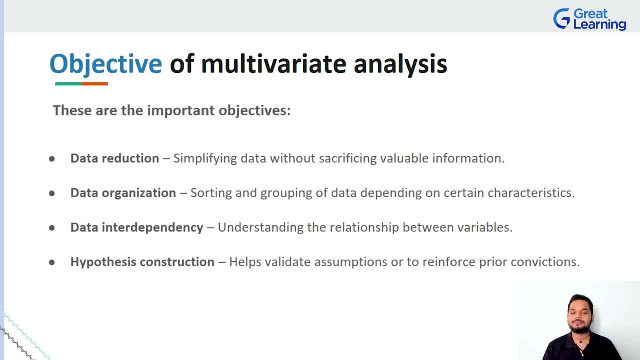 so again, whenever you're thinking about all of these things, it is very, very important to first of all analyze. when you say data analysis, it's not just taking a data, analyzing and giving something out. there is way more sophistication to it, as you can see on your screen, and this is very 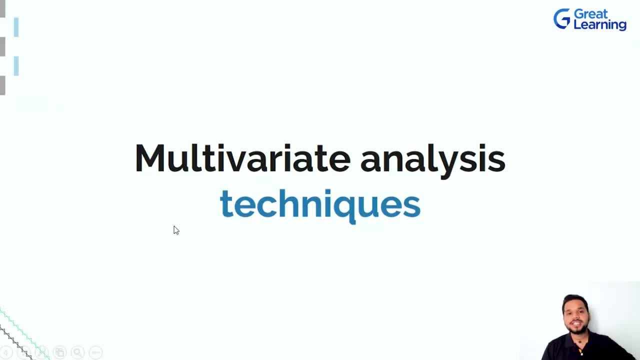 important for all of you all to understand. all right now that we understood the various objectives of multivariate analysis, i think it is high time we dive right into the heart of the topic to actually understand what are some of the various techniques that we have in today's world. 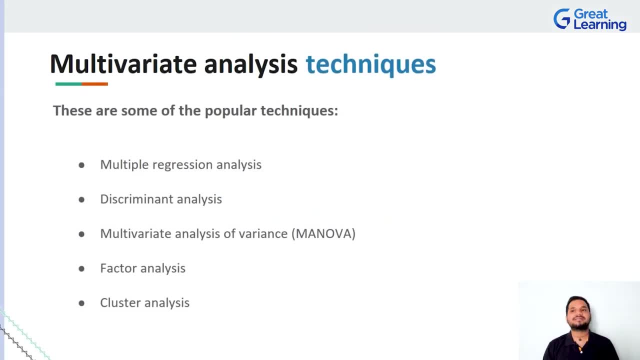 to help us with multivariate analysis right now. ladies and gentlemen, there's many, many techniques of how one can go on to perform multivariate analysis and, as a data analyst, it is very helpful for you to know what each and every one of these techniques are and how you can perform multivariate. 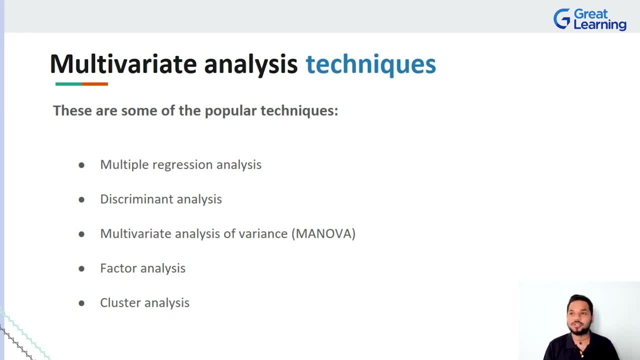 analysis is now. a common question i get whenever i'm teaching these techniques is: do we have to know all of this to an extreme amount of detail? not really, because whenever you you given a problem statement, you will be using various techniques out there- let's be honest. but it 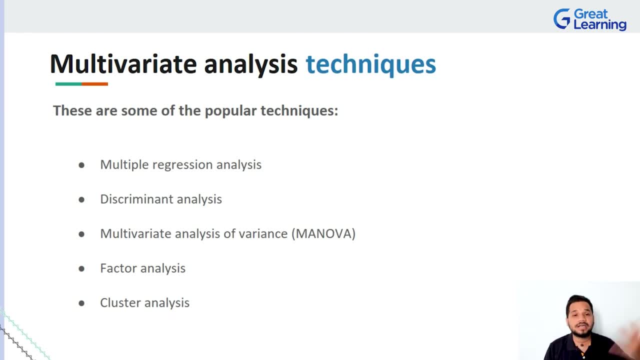 doesn't add any sort of value for you to be a thorough expert in 100 different techniques when you might be just using three or four. right, give it a thought. so, whenever you require any sort of technique, know what it is, know where it is used, know this. uh, it's very important for you to. 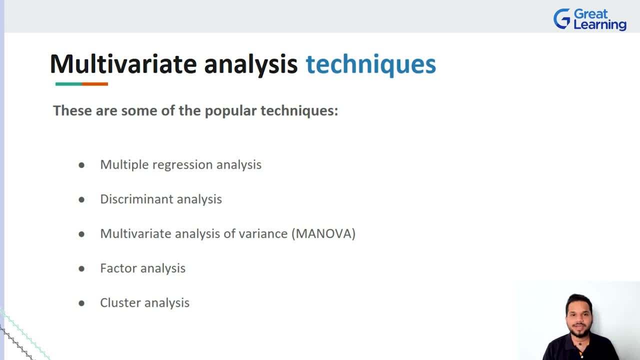 understand how to use the technique to solve the problem. that is where all the uh magic lies in right? so let's quickly brush through, let's quickly summarize some of these really popular techniques that we have in today's world. uh, where multivariate analysis is popularly performed, right, 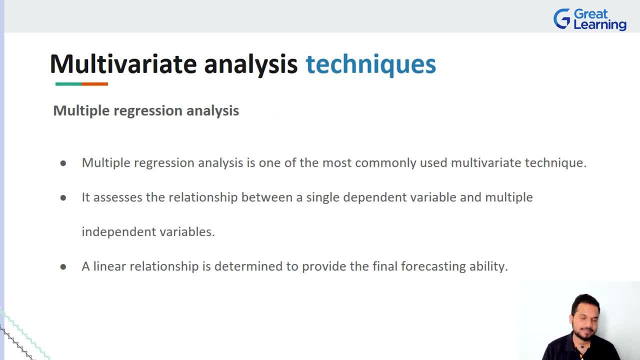 the first one on your list is multiple regression analysis. multiple regression analysis, or mra as it's called, is again one of the most commonly uh used multivariate techniques out there. why? because it is uh. it is very effective even from a non-technical perspective and, at the end of the day, when you're performing multiple regression right, it just solves all of 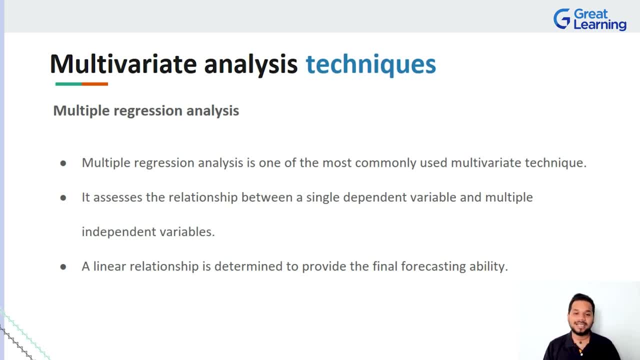 your problem because it will help you assess the relationship that exists between one single dependent variable and multiple independent variables. are there? there is one single dependent variable. there's multiple independent variables around it. so if there's any sort of relationship that exists, this analysis method will show that out in bold to you right. so when you have this, 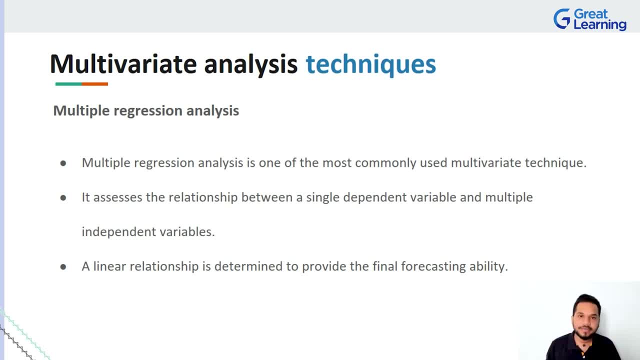 kind of an ability where you know you have one dependent variable, multiple independent variables, you can determine a linear relationship very, very easily and eventually to- let's just say we're trying to use this technique to predict tomorrow's weather. it's going to be very easy. what is the goal? 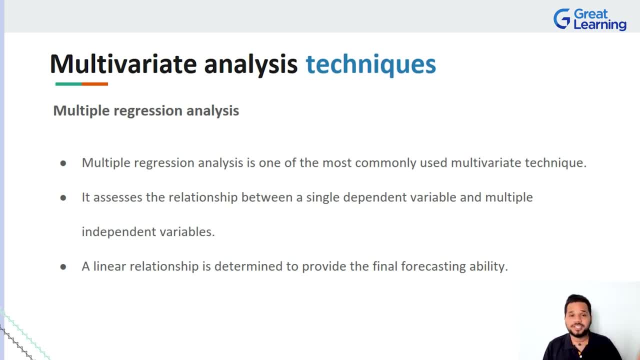 here, the weather. what are the parameters that will help for the weather? uh, precipitation, pollution, uh humidity, all of those factors, right? so you're building a linear relationship between that and once you go on to actually do it, well, you can, you can predict tomorrow's weather, right simple. 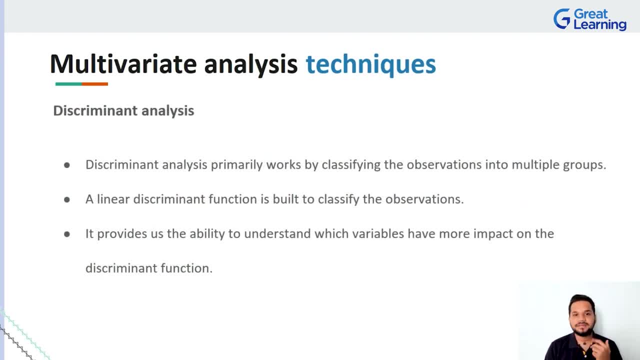 that is, multiple regression analysis. now coming to talk about discriminant analysis is again another very popular multivariate analysis technique. but here, uh, what we, what we do. things are slightly different here, because what we're doing is we're trying to classify all of our observations and we're just creating multiple tiny groups, subgroups, bunches, whatever you want to call. 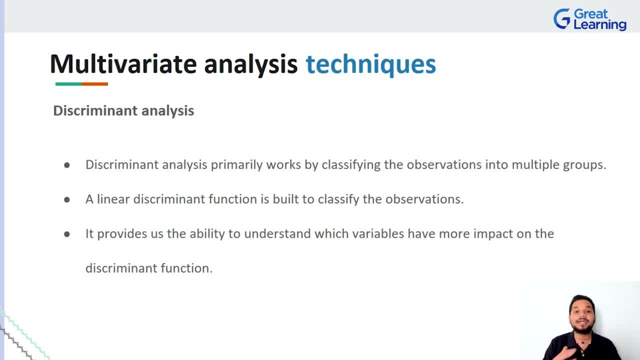 it right. so we just take all the observations and we split it out into different groups. now we can have a function that is, that will basically classify all these observations that we have right now. once you have observations, you divide it into groups, you will know roughly what the 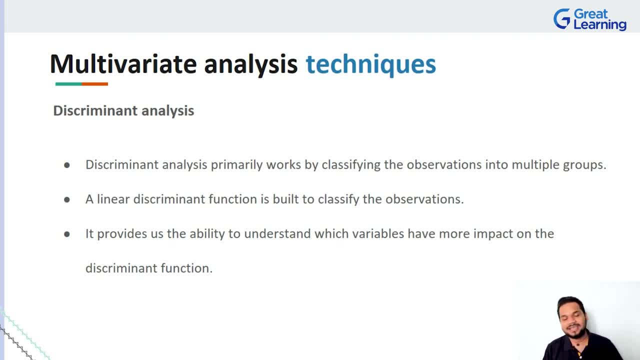 vaguely what each of the groups or how each of those groups will behave, and then writing a function on it to make sure that you can. you can sit and classify the observations for sure you're no longer guessing. you have a structured way of actually performing that assessment. you can do it. 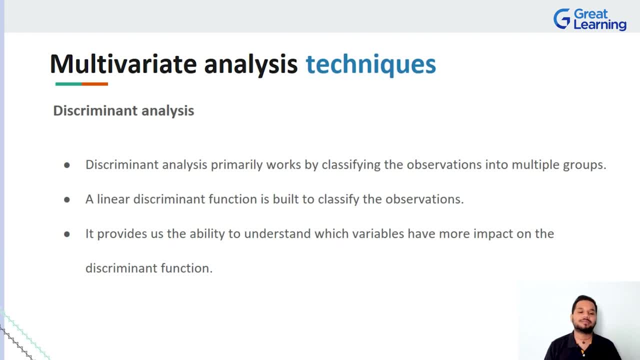 right. so it will give you this ability to understand what variables will have more impact on the function at hand. now again, think about the diabetes example that i've been talking about, right, how do you know which has the biggest factor? does having really high blood pressure cause diabetes? 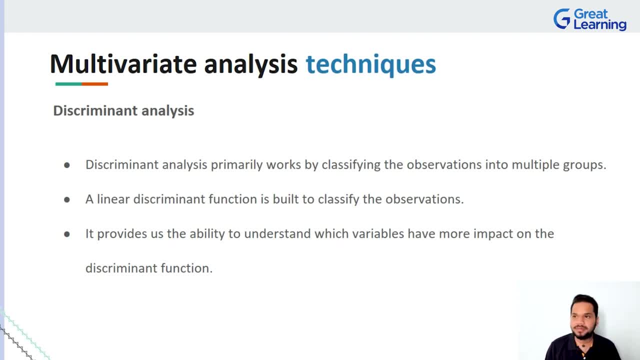 having, uh, really bad blood sugar levels cause it. you know, you cannot say you have a bad age or something. uh, you can say maybe you have a bad body mass index. right, personal fitness maybe, if that isn't up to the mark and if you see if you are obese or very obese or something like that. 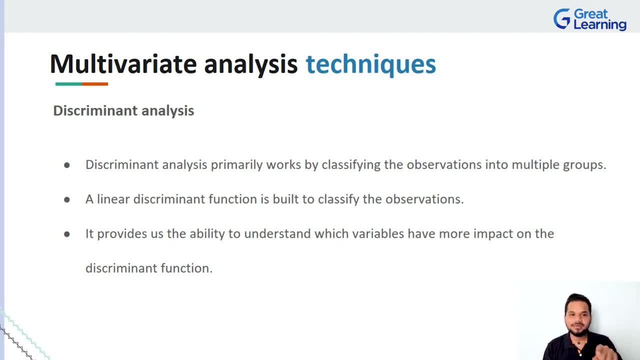 how do you know which of these has the highest impact? right, using discriminant analysis, you actually have the ability to say, hey, this uh particular feature, this particular uh point of analysis, might have that much, that much an impact on your solution, and that is very, very important for you to analyze as an important. 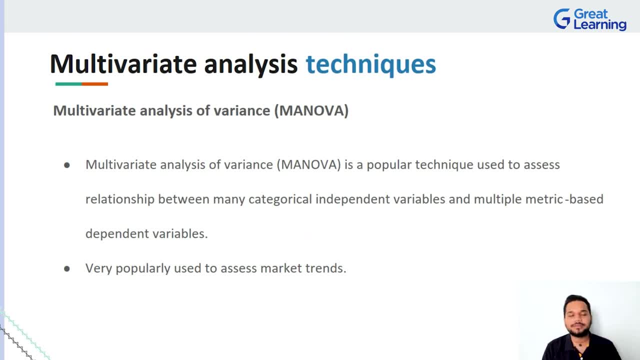 technique we have today, right, and then coming to another multivariate analysis technique which is super popular, which is basically called manova. manova or multivariate analysis of variances, again a super popular technique which is used to assess the relationship between- note this: this is used to assess the relationship between many categorical independent variables and multiple 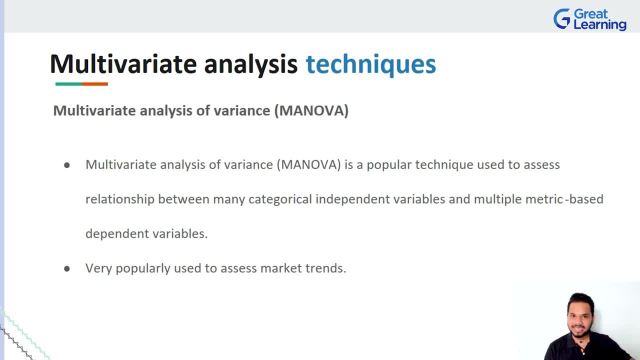 numerical dependent variables. independent variables are categorical- uh. independent variables are numerical. right now, when, when, this, when is this the case? give it a thought, right? i actually want you guys to analyze. when is the situation where you will have a categorical independent variable and a numerical dependent variable right? uh, it will give you uh to give you. 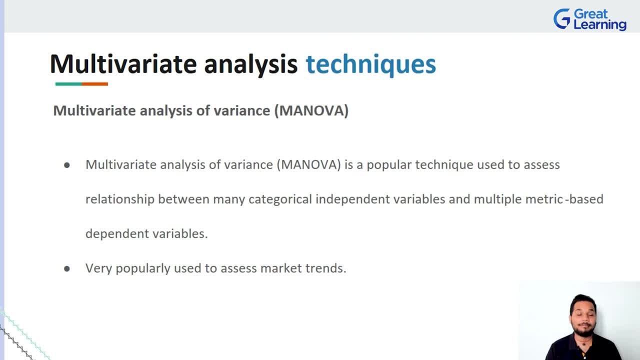 a hint to take a look at it. it's very popularly used to assess the market trends. we know how the market works. right, it's just charts up and down. but when you have to analyze how much something is very dependent from a numerical dependent variable, anyone will get more waits to turn. 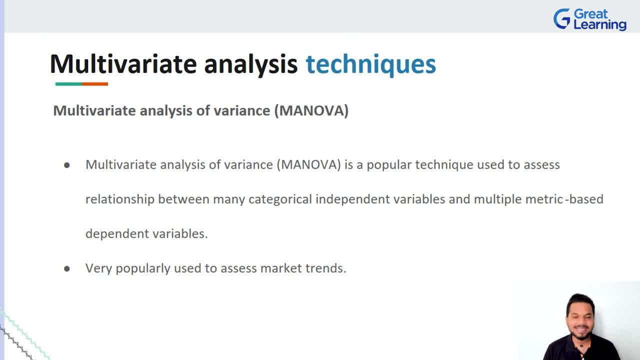 it on, but when you see a very cat SOFT than the more dependent. that is essentially what people varying with respect to another point, you're going to have to take a look at the variance and once you have to perform analysis on the variance and if you have to perform multivariate, 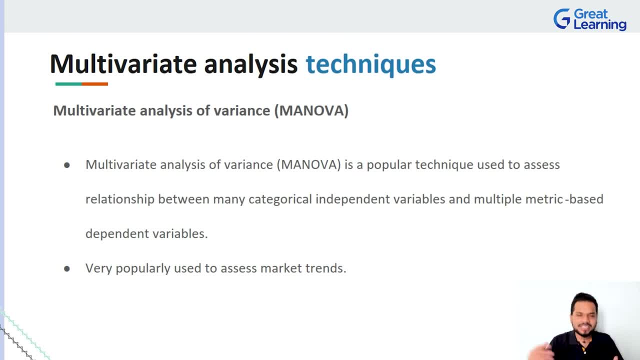 analysis of variance. it's called as manova right. it's a. it's a very simple generalization of what the technique is, what the technique does. but this point where it says this is the relationship, it will help you assess this relationship between, uh, many categorical independent variables and 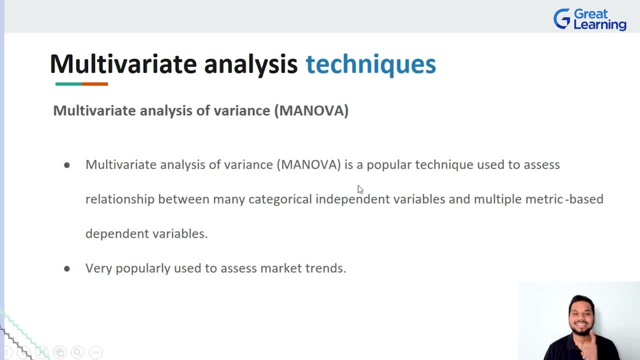 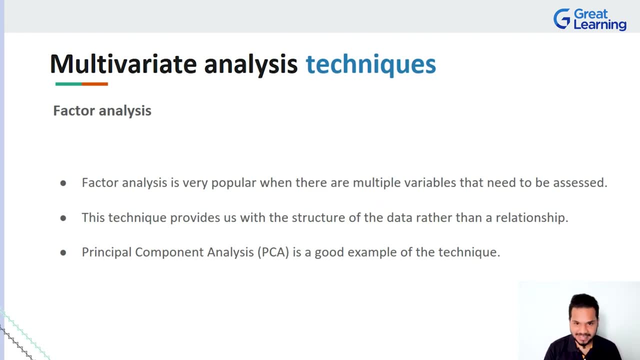 and, uh, metric based dependent variables. this is something that you guys should understand right. coming on to the next technique, which is factor analysis. right now, factor analysis is also another very, very popular technique. now you might be- uh, you know- taking a look at the trend here. i'm 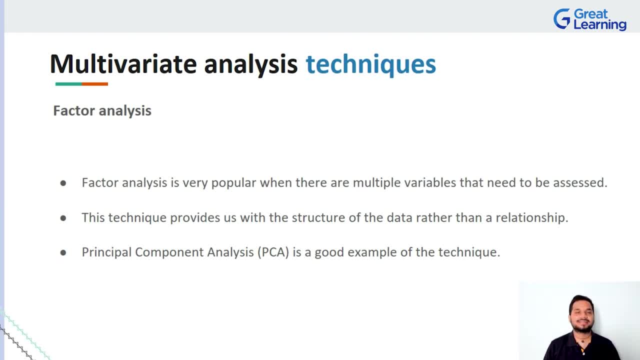 saying that this technique is very, very popular because data analysis is such a huge domain out there. each of these techniques have become popular because they are very good at solving certain problems for multiple domains out there right now. factor analysis is very different from all the various other techniques that we have today because- see in the other techniques that you will 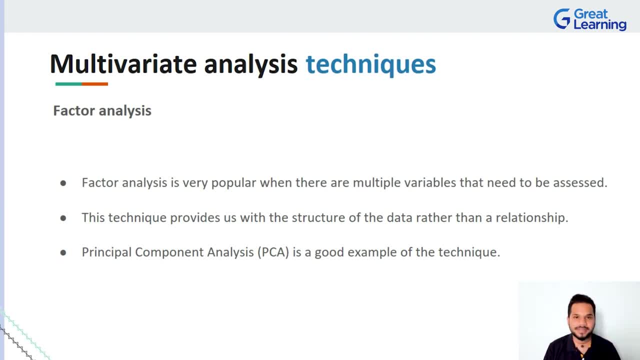 have you will. we're trying to find relationships between variables- right, dependent, independent, categorical, numerical, all of that- but here what we're trying to do is we're trying to understand the structure that is hidden in the data, rather than say, hey, i want a relationship and, uh, you. 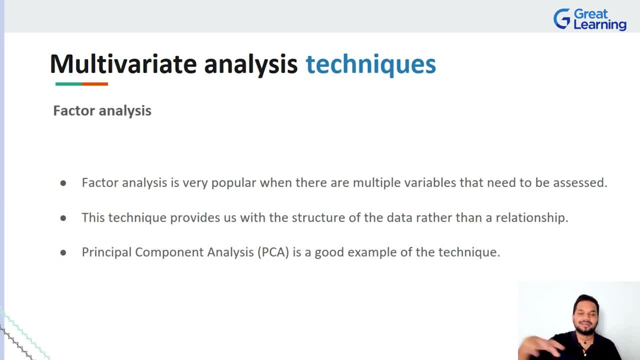 know, when i say i want a relationship, basically i mean the data, uh, point, uh. you know finding relationships between each other right now. that is very important for you to understand. and i bet you have heard about factor analysis, right, pca, principal component analysis. i'm sure you. 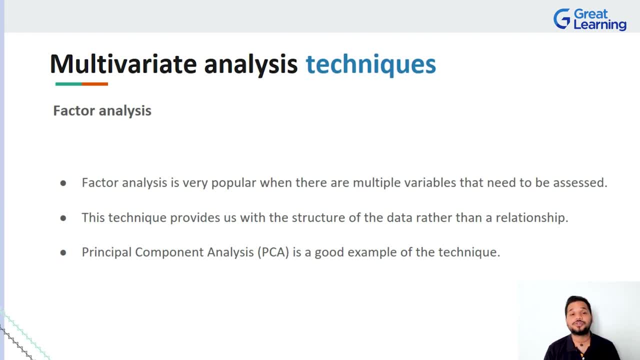 might have read about it, but i'm not sure if you have read about it, but this is a great about it- heard about it or something- and in fact, what you should know at this moment of time is that pca is a very, very good example of actually performing factor analysis. a point where you say: 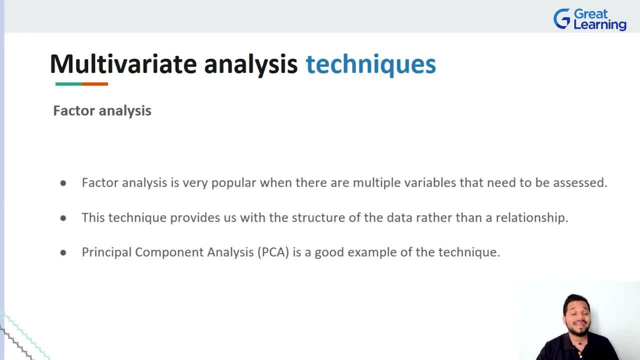 hey, i want to understand the structure of it. i want to understand why the data- uh, you know why the variables behave the way it is, and how is it linking to each other. when you are hunting for that structure, rather than just looking for, uh, for looking for the relationship between the variables, 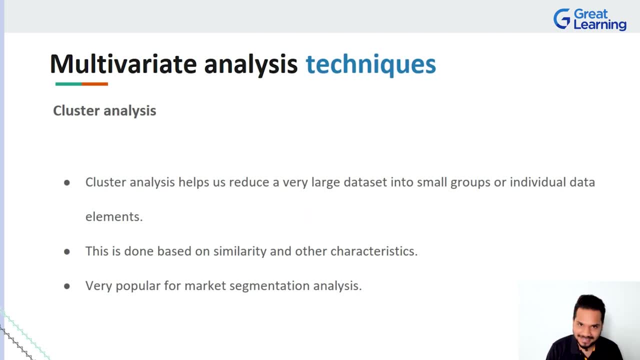 you know what to use now, right, factor analysis. and then we have another type of- uh, multivariate analysis technique here, or it's basically called as cluster analysis. now, cluster, what does the name cluster remind you of? right, because in this particular case, when we are performing cluster, 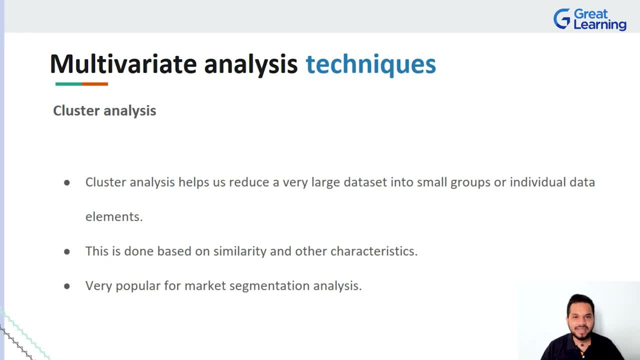 analysis. we take a very, very large data set and we actually break the large data set into smaller chunks, smaller groups of individual elements, right when we are performing cluster analysis. that's what we do: we take large data, we cut it out and small pieces and we analyze those small pieces and we try to understand: is there any sort of 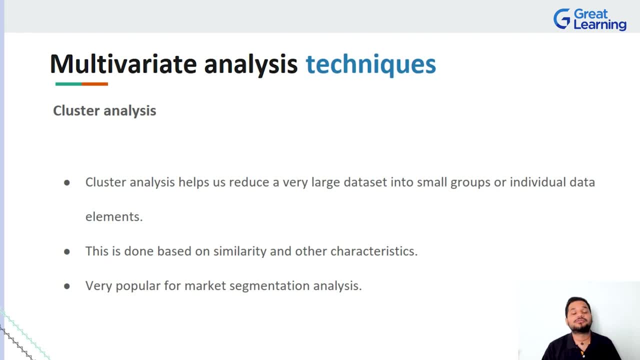 similarity when we're trying to cluster this. is there any other characteristics which will group it into clusters? right, i'll give you an example. think about apples, right? uh, if i the fruit apple, not the brand. uh, now, whenever you're thinking about the apple fruit, there are so many ways. 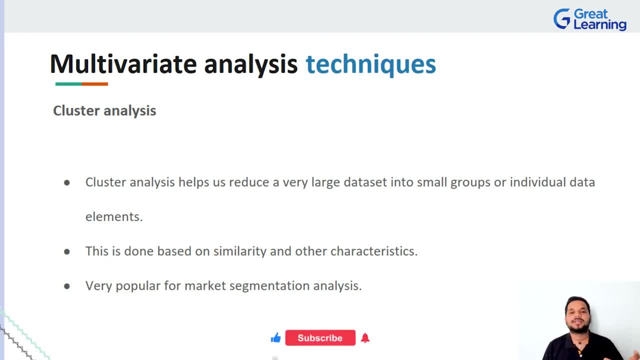 there's a, there's a raw apple, there is a ripe apple, right, the raw apple is usually green in color, the ripe apple is usually red in color. now, what if i say, hey, can you, can you divide this, can you cluster these apples based on if they have, uh, if they've ripened or not? what will you look at? 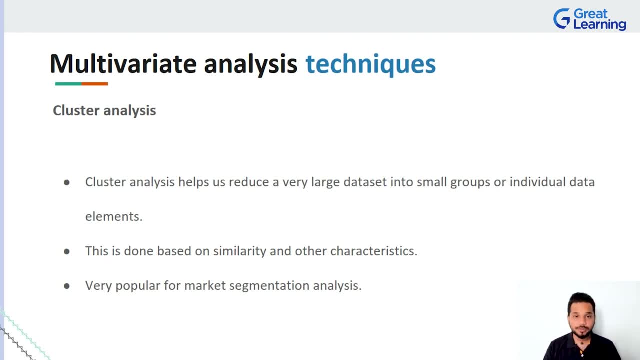 you look at the colors, hey, this is green, unripe, this is red, ripe. you're going to do that right. so it's a characteristic that you're trying to assess. similarly, when you have so many different things, especially market segmentation analysis, uh, where you will have a lot of these categories, where you 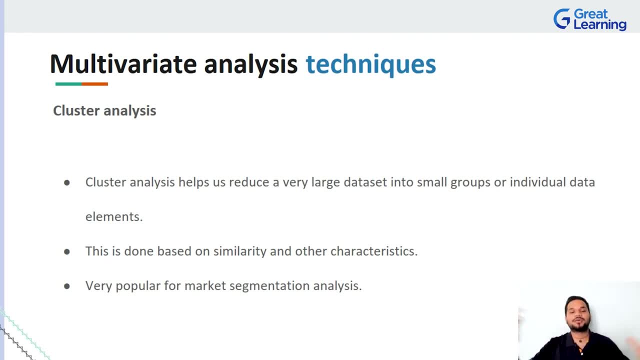 know your data is huge. it's absolutely huge, but you can, uh, try to group it down, try to simplify it and understand. hey, these are similar points of data that i can club. these are some of the mistakes which are making the data points look similar, so let me club these as well, right, and? 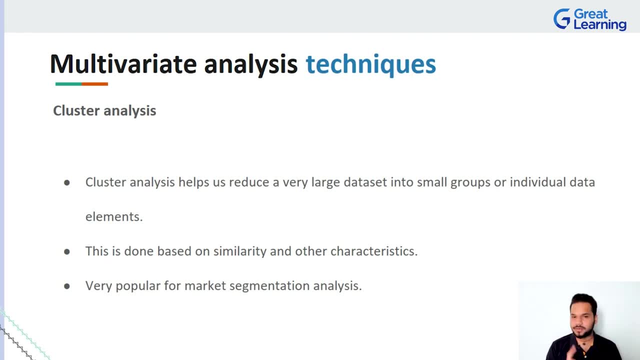 then later you perform analysis on it. how simple is that? but you have to understand one thing, ladies and gentlemen: uh, factor analysis and cluster analysis, as we are discussing right now, these are very, very popular, very powerful and uh, people have started to realize that it is way it pulls. 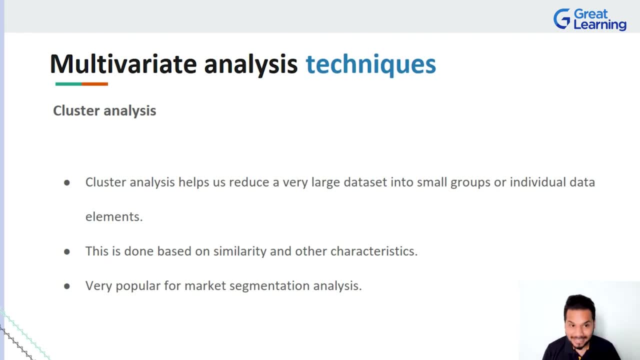 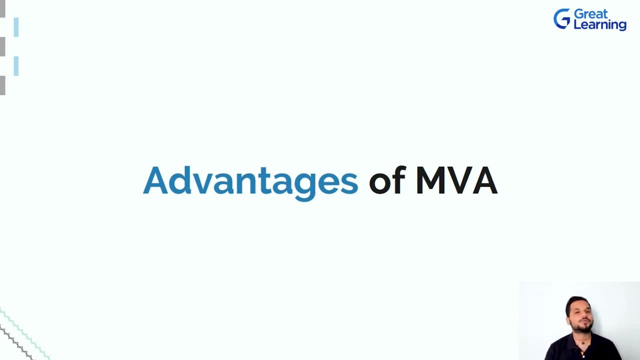 way more weight than people initially thought, so these are extremely popular. uh, for today, right, the next thing that we're going to take a look at some of the various advantages of multivariate analysis that we can have today. now to talk about the advantages of multivariate. 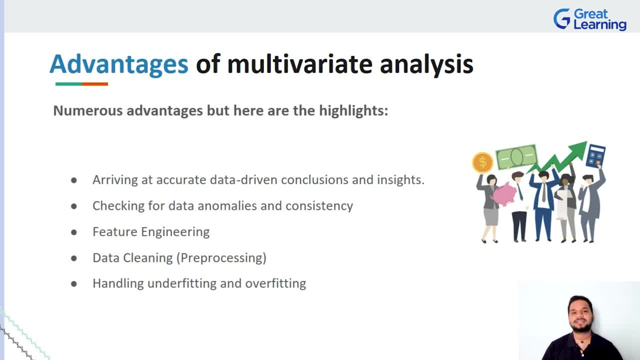 analysis is a small problem, because there's a ton of advantages that you can talk about right. there's huge number of advantages, which i can go on and, on and on, but to actually simplify all of my thoughts into five, six very good points, that's what you see on your screen right now. the biggest advantage of 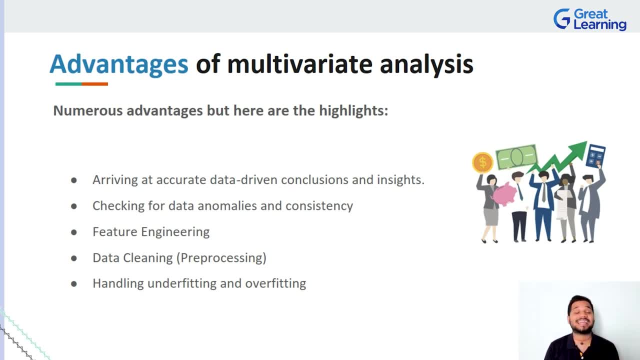 multivariate analysis is for a fact, that it will help you arrive at accurate, data-driven conclusions. so you can come to a conclusion, one, you can guess it, the second one, you can have a conclusion and you can say: i have data to prove that this is the conclusion. which would you pick if you were a 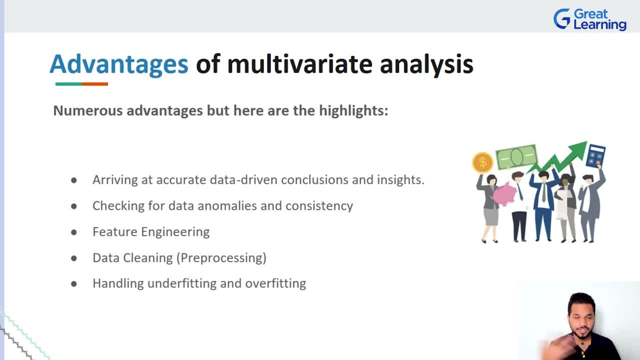 client. if you were an individual, if you're an enterprise user, which would you pick? you would, of course, want data-driven insights, data-driven conclusion. it will help you arrive at that right: not just data-driven conclusion, but accurate, super accurate data-driven conclusions right now. the next point where multivariate analysis actually helps is to find out if there's anything wrong. 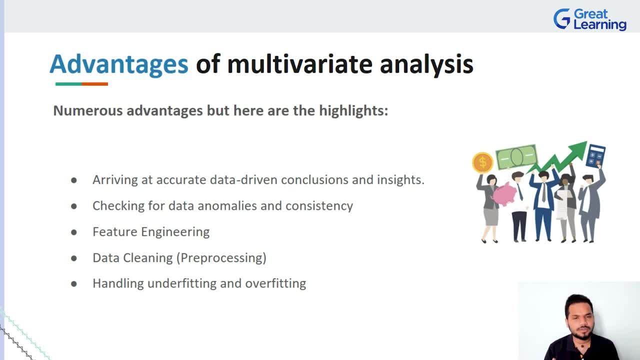 if there's any anomalies in the data and also to understand if- uh, to understand what, how level of what is the level of consistency that you have with respect to data out there right now? this is very, very important for all of you all to understand, because people usually think that hey. 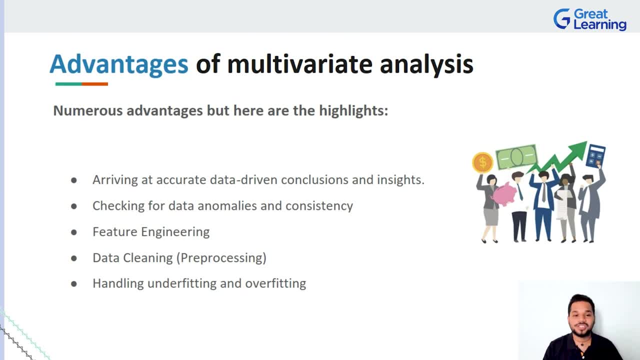 multivariate analysis. you have multiple variables, you analyze it, you give some conclusions, you're done. not really it'll help you in a lot more places. think about the third point: feature engineering. feature engineering is actually a concept where you will try to analyze what parameters have what. 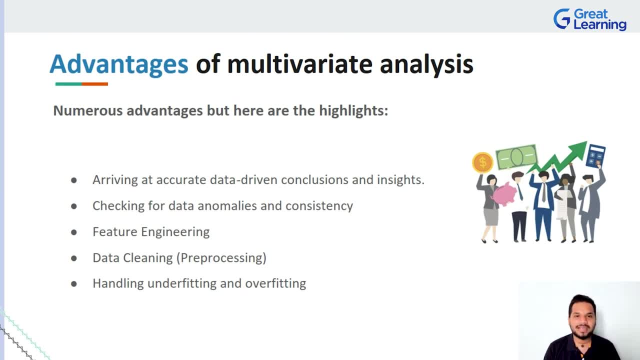 kind of impact on your outcome, very similar to multivariate analysis, or in fact, it's an initial step to multivariate analysis, if you take a look at it from another perspective as well. so telling that, hey, these are the features which will help me. age is a feature that will help in diabetes. 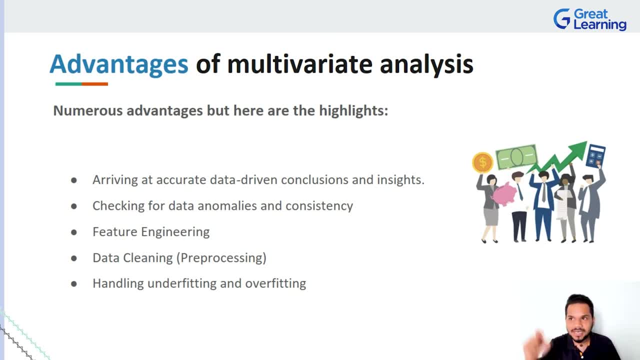 uh, genetics is also a feature that will help in diabetes, right? so you have multiple features that you're going to say that this will uh have, uh, you know an outcome. this will have an effect on the outcome, right, that helps. again, feature engineering is extremely critical, critical. 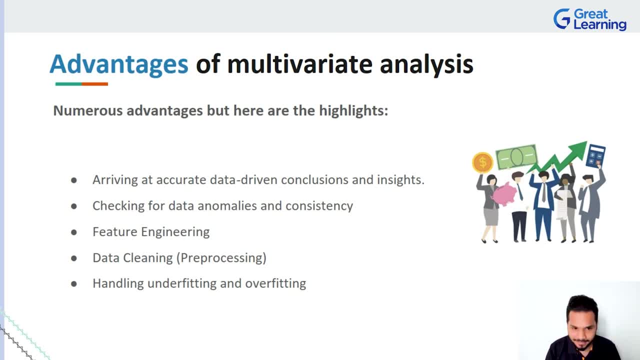 learning. so give it a thought of how, how advantageous this is right. and then data cleaning. data cleaning is very, very important because, at the end of the day again, if you consider a machine learning application, if you- uh, you know, if you just provide unclean data to, 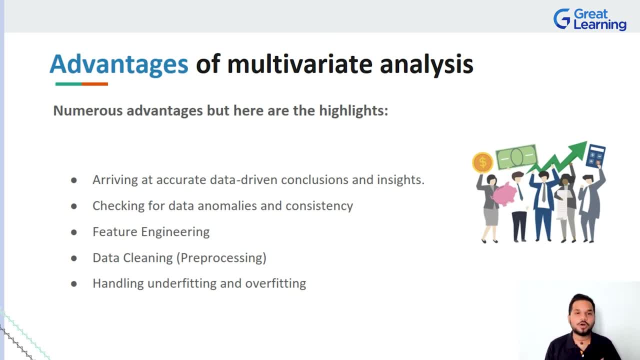 a machine learning algorithm. it is not going to realize. it doesn't know what a car looks like. it doesn't know what a ball looks like. it has absolutely no idea, right, it understands only zeros and ones and through structure it builds and understands and has a certain meaning. but 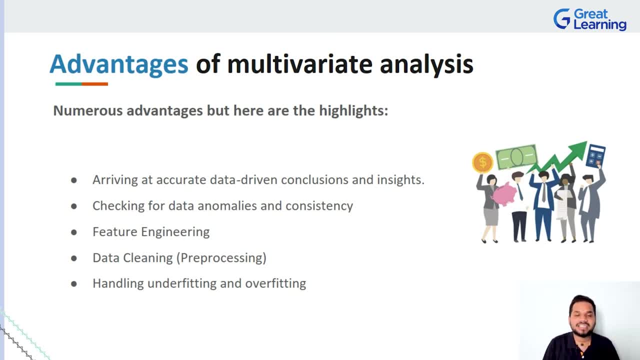 your data is unclean. uh, let's just say you're trying to collect the patient data. someone has asked: what is your blood group, right? so some person by mistake, instead of typing in their blood group, they have written their date of birth or they have written their mobile number, right? 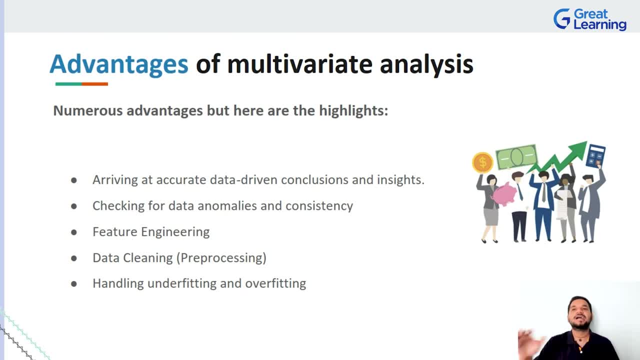 think about it. it can happen. it will happen, right? we're humans, after all. so when something like that happens and when you know that, uh, you know the data data is incorrect, and as soon as you feed it to your machine learning algorithm, it doesn't know it's wrong, what it's going to do is it's. 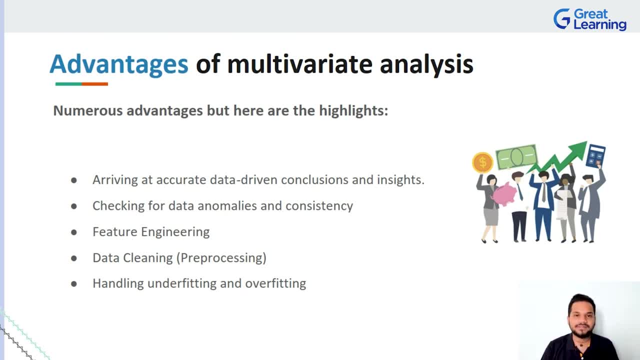 going to use that to learn incorrectly. right, it's not its fault at the end of the day, but it happens. so, with respect to using multivariate analysis, where you can clean and pre-process your data better, helps a million folds for all the processes which come down the line after analysis. 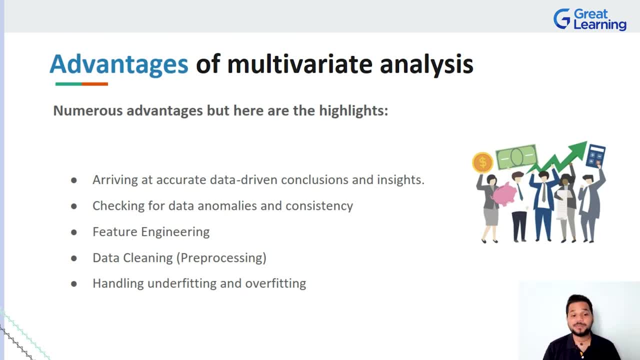 right, superb, take a look at the last point. the last point says handling underfitting and overfitting. underfitting and overfitting are the absolute. you almost feel like, hey, these are small problems, but these are the biggest impacts on the outcome of whatever is being done. 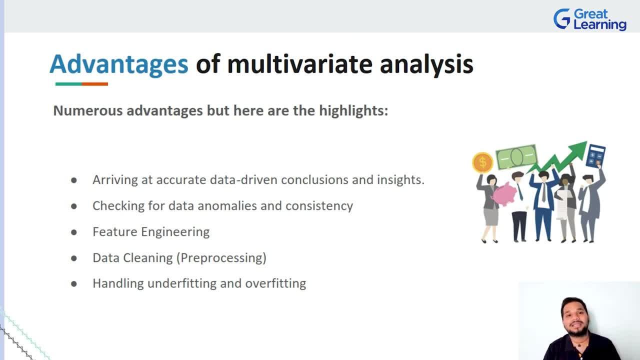 right. underfitting is when your machine learning model cannot really, uh, go into the depth of analyzing and assessing- uh, what's going on with the data? so it really cannot dig deep enough to find out any structure pattern or anything. but overfitting is reverse overfitting. it has dug so much into your problem, it has dug so much into your data that, instead of 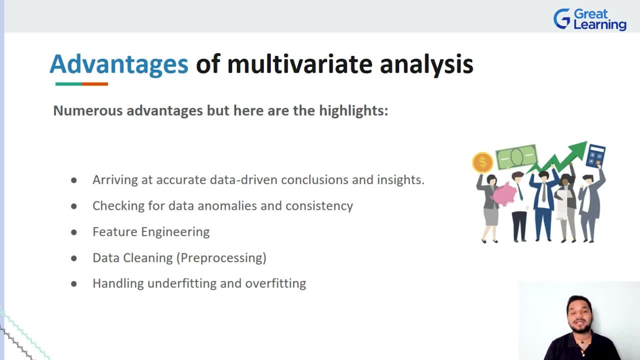 looking at useful data. it started looking at noise. it has it started picking up things which are, which might be of no use, uh, to your outcome. and what does that do? that, both in underfitting and overfitting, it ensures, at the end of the day, your overall performance is coming down. your machine learning. 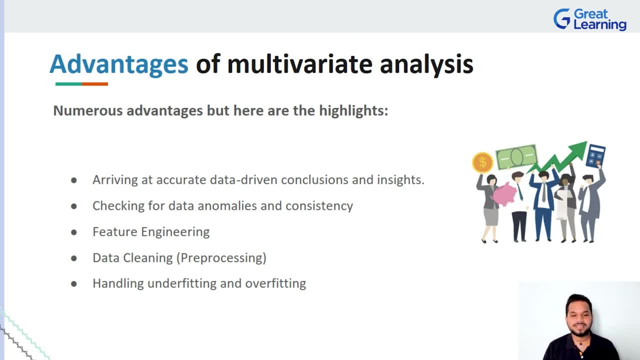 model is not going to be performing well. why? because it's doing all of these things right one. in one case, it has absolutely no idea what sort of data to pick up and work on where. in the other, uh kind of case where it's working so hard at a granular level that it does not know it is not. 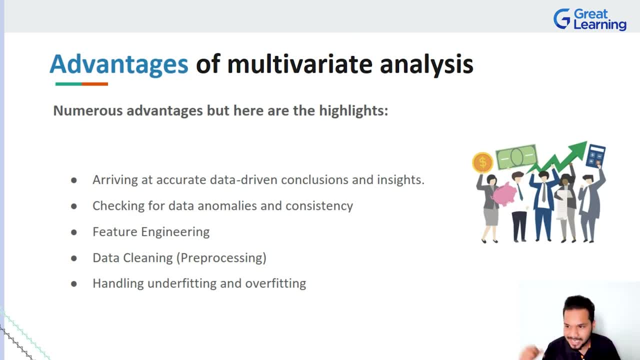 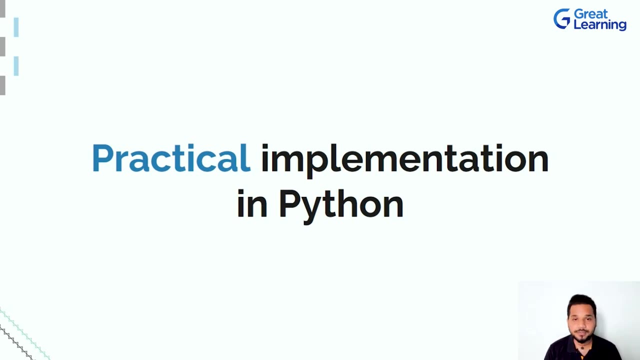 able to differentiate between noise and it is not able to differentiate and it is not able to pick up anything useful in both the cases, right. so to avoid all of that, to help handle it again, you have a point wherein we can actually take a look at that fantastic diabetes demonstration that I just 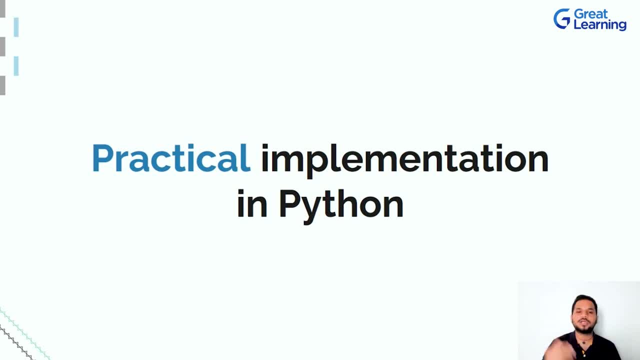 mentioned to you all, and let me quickly jump to Google collab. Google collab is nothing but a Jupiter notebook that is hosted on the Google Cloud platform. now you guys can code this in any other- uh, you know- any other choice of ID that you want. your pie charm, you can use the regular. 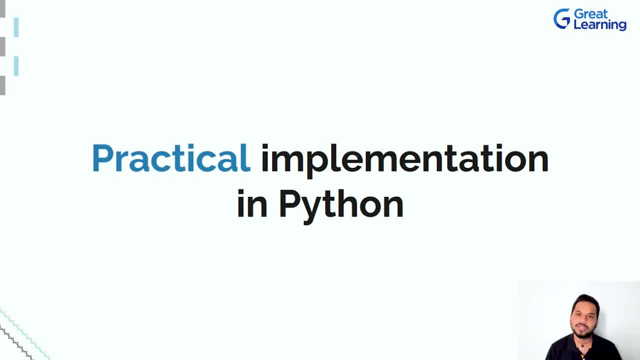 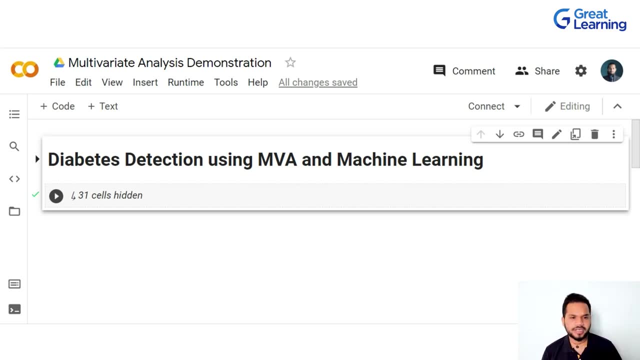 Jupiter notebook. it's basically a simple Jupiter notebook, but it's on the Google Cloud, right? so let's quickly get into that. all right, guys, as you can see, I've opened up my Google collab out here and all we're trying to do is we're trying to perform the diabetes. 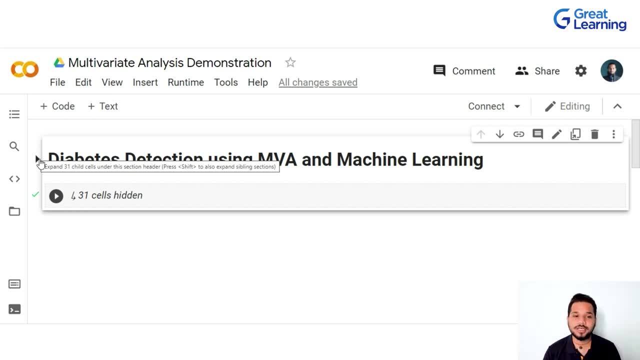 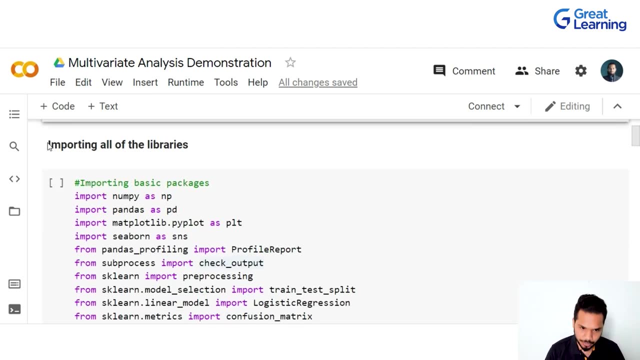 detection. we're trying to understand how we can get a machine learning model to figure out what are the various factors, what are the various points of analysis that will eventually lead uh to the result. right, uh now, ladies and gentlemen, the goal here, one thing you have to understand, is: 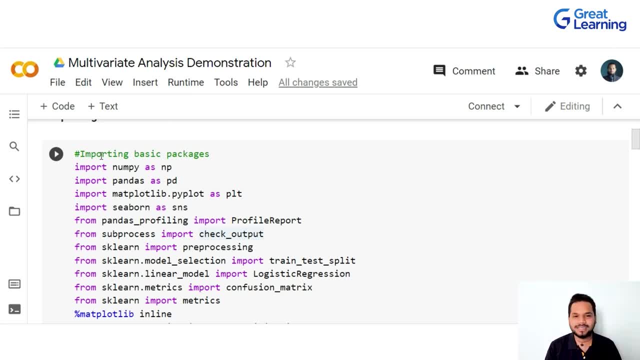 that the goal here is not to show you how easy, of course, one point: you have to understand that to achieve, uh, this particular demonstration, it's very, very easy, but I understand that some of you all might not be, uh, you know, might be able to understand that. you have to understand that you. 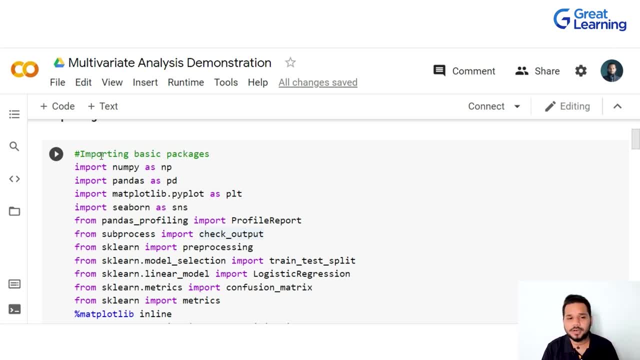 might not be up to speed with respect to these libraries, such as numpy, pandas, matplotlib, seaborn. so let me quickly give you a glance of what's happening with respect to each point of code. but you actually try to analyze and assess the uh, NVA- the multivariate analysis aspect of it- right well. 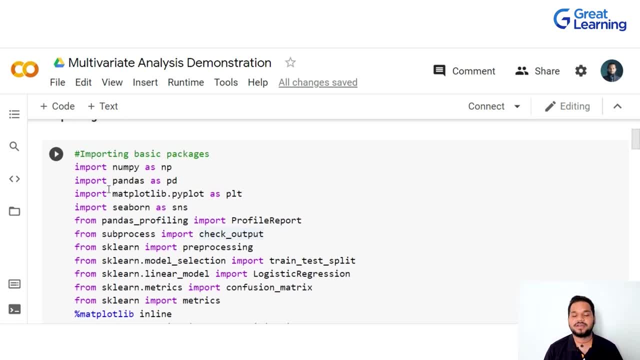 the first step of any analysis out there. uh, we're going to be have, we're going to have to import all the libraries, right? numpy is called as numerical python. it's basically used to perform all these numerical related activities when we are working with python. pandas will give us two fantastic data. 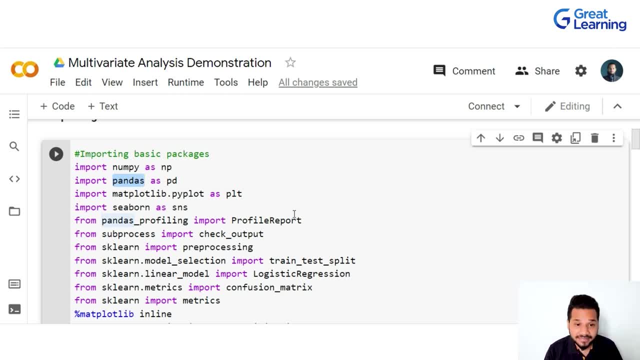 right, it's called as, uh, the pandas series and the pandas data frames, which are again very, very important for us to work with. and then we have matplotlib and seaborn. matplotlib and seaborn are critical libraries when it comes to data visualization. if you have to plot anything, uh with. 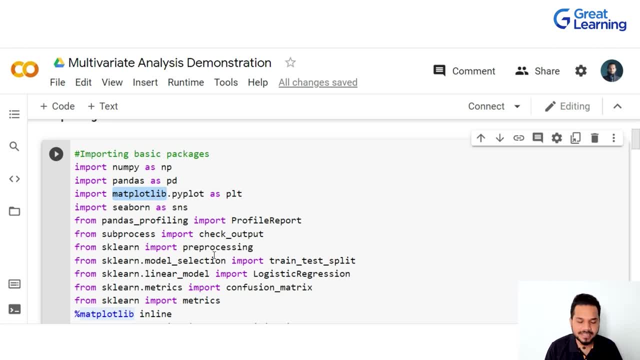 respect to using graphs, charts and all of that which we are going to be using in this small demo. so you're going to require that. and then we have sk learn. sk learn also stands for scikit-learn, which you might have heard. it's a very, very important library for machine learning right now, as soon as 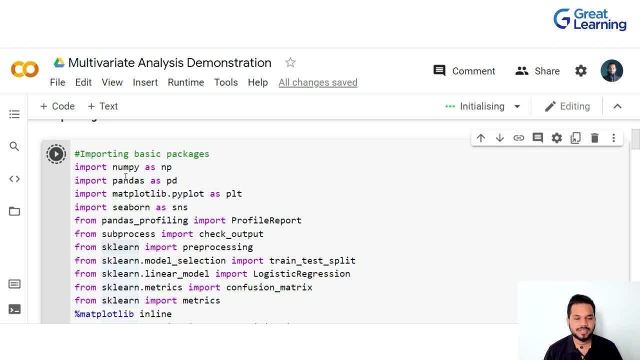 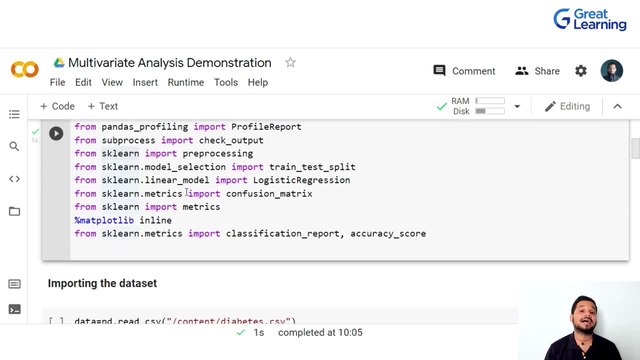 you're using it. it's very simple to actually work with uh, Google collab here now. as soon as I hit the play button, it's going to take a second and as soon as it stops, basically it has executed this. right now, all these libraries are ready for me to use. now the next step is for me to actually talk. 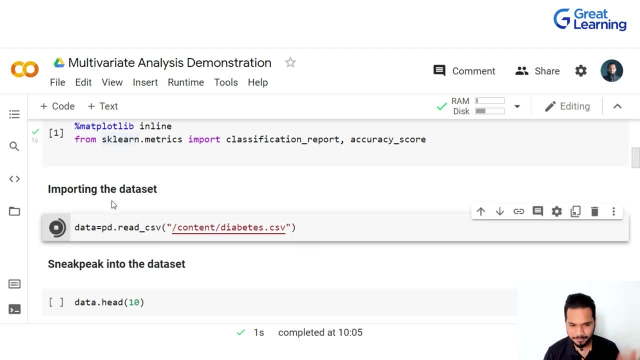 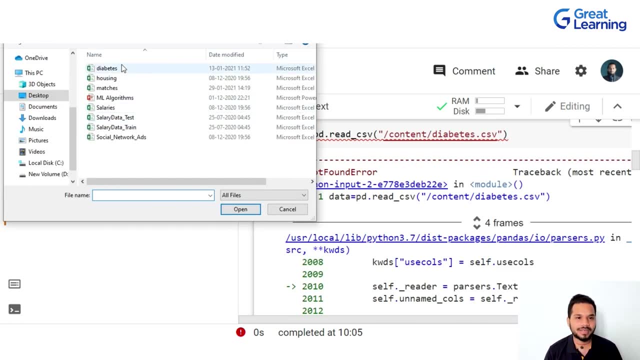 to you about the data set right to show you what the data looks like. but if I just hit play on it, it's going to give me an error. now it's going to say, hey, where is that file that you're asking me to open? well, it's actually in my local computer here. let me open up these files now. I have to. 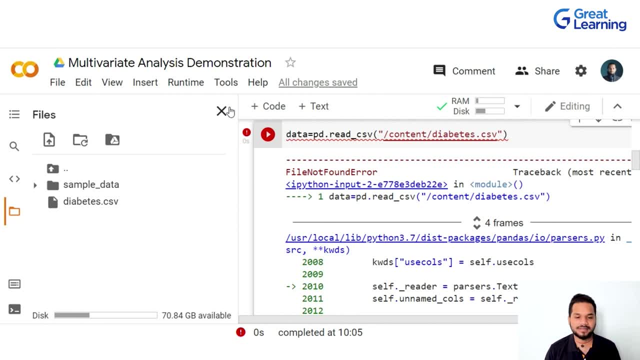 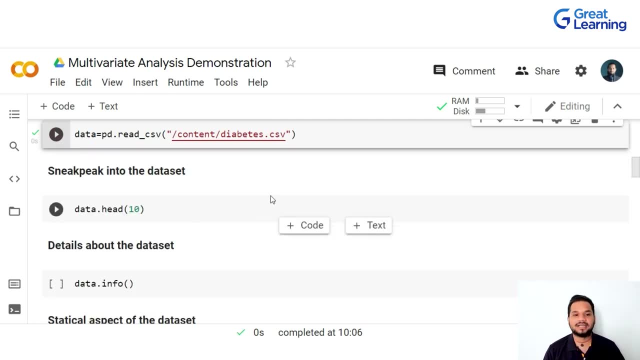 upload it to the Google Cloud so that it understands. right now, this entire python environment is on the Google Cloud. now that I've uploaded it, I'm going to close it, I'm going to hit play again and as soon as I hit, play again: done, we have. 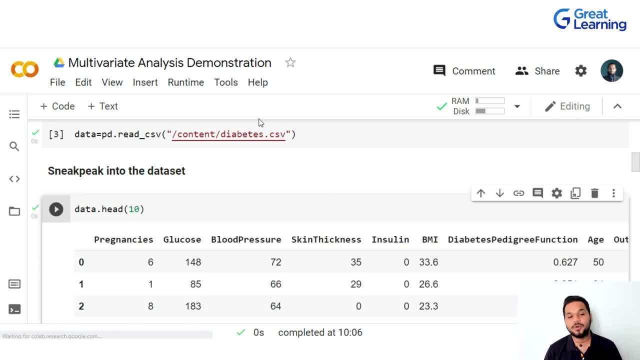 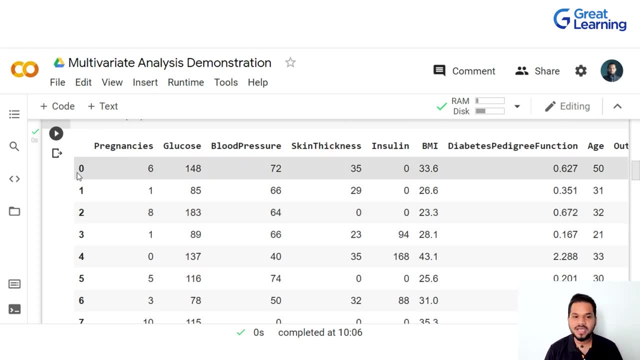 actually uploaded our data set. our data set is ready, so let's quickly take a look at what the data set is all about now. now I've printed the first 10 patients worth of data. now every uh row you see here is one patient's data. okay, so we have multiple uh ones. we're gonna see how much. 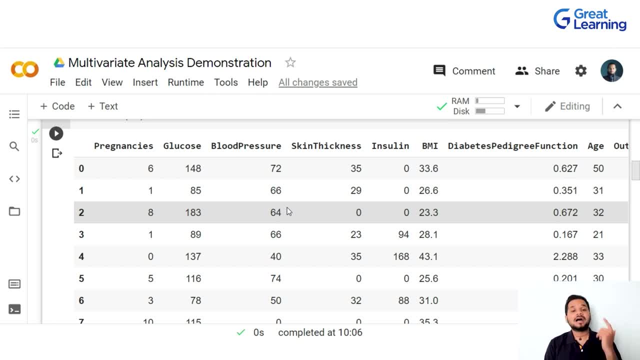 uh, that cause diabetes, right. one is your glucose level, uh, the blood pressure levels. what is your skin thickness? what is your insulin level? what is your body mass index? what is your age? and eventually, the last column will be the outcome column. right now, if the outcome is zero, uh it. 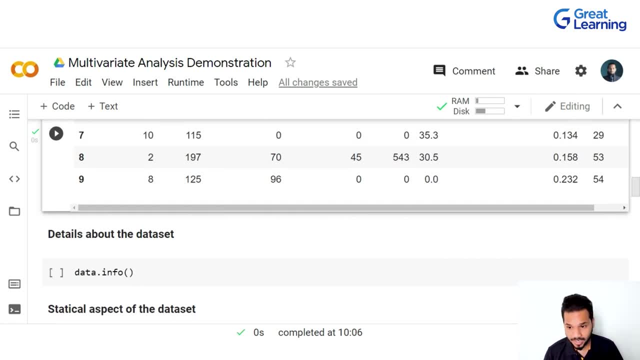 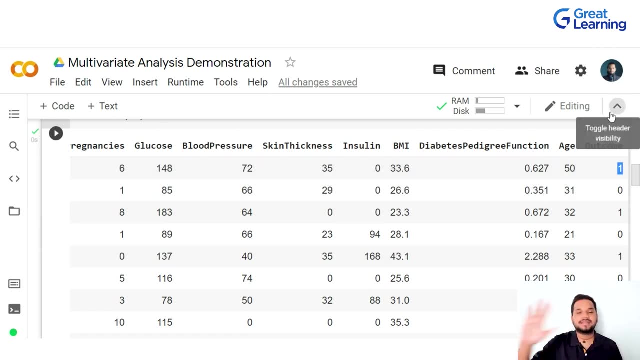 means this person does not have diabetes. if the outcome is one, it means that person has been diagnosed with diabetes. right? so we already know. we know that, hey, this is the detail of the person who has diabetes or not. we know. but what we are going to do when we are supplying the data to our 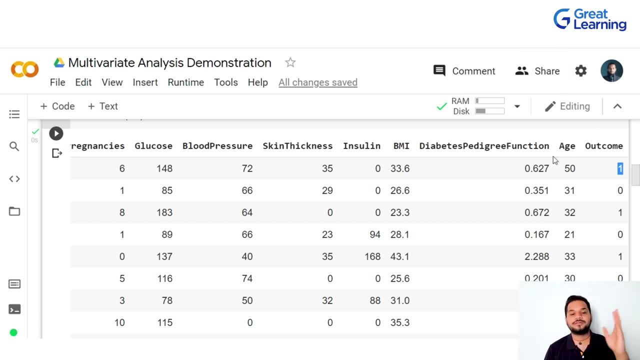 machine learning model is we're going to just remove the last column and say, hey, now you predict if there is any sort of uh. use your multivariate analysis result to see if you can find out correctly if the person has diabetes or not, right? so that's about it. uh, BMI again. when you think. 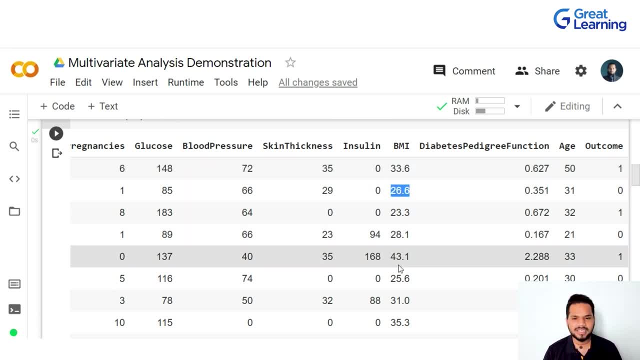 about it. I think 25 is the normal value. anything about 28 or 30, something is where you are called as an obese person. anything less than 25, uh, you know, if it is like around 20 or something, your mall, new malnutrition or something along the lines of that, right, you guys know this. now the important part. 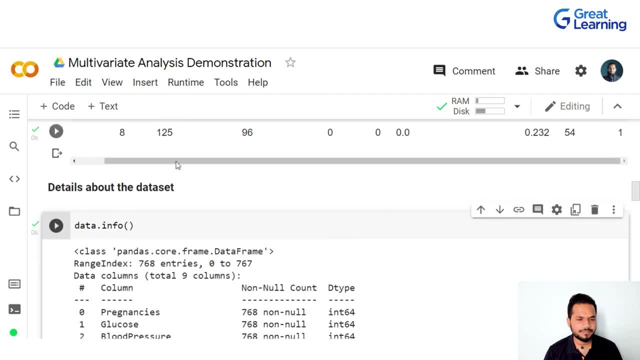 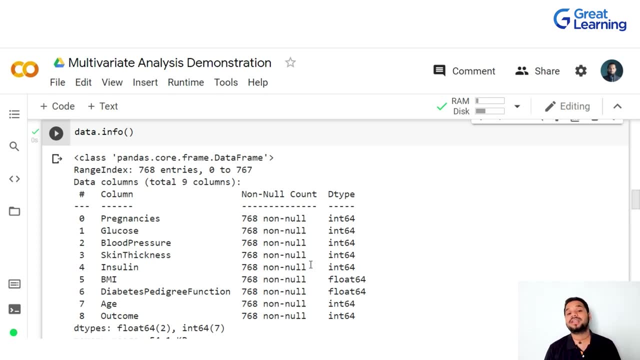 that you, you have to be asking me right now is: hey, okay, so you just printed out it for the data for 10 people. how many people do we have in total to analyze all of this data? as you already know, to perform multivariate analysis, we require a large amount of data, correct? yes, in this case? 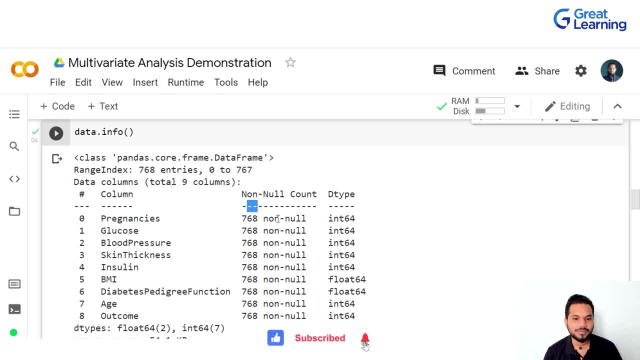 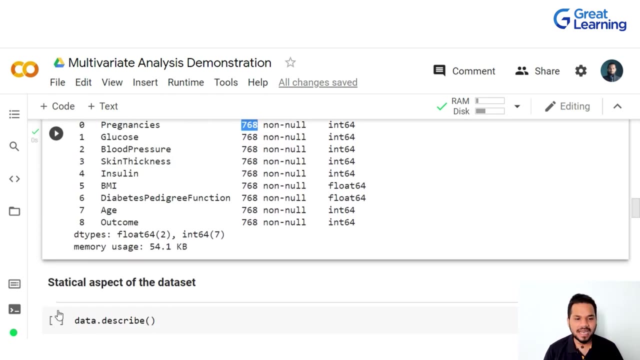 as you can see, for each of the patients, for each of the columns that we have, which is showing a parameter, which is showing a variable, we have 768 entries. what this tells me is that there are 768 patients worth of data that I'm looking at right now. okay, so if there are 768, 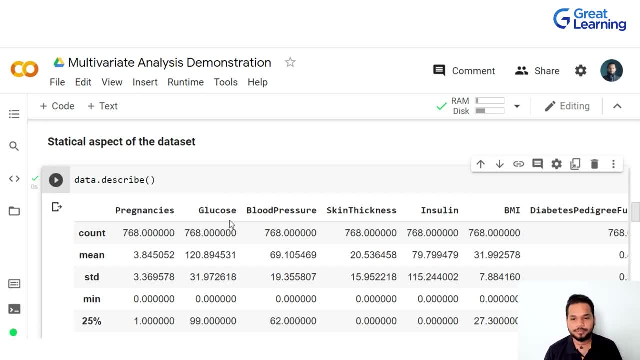 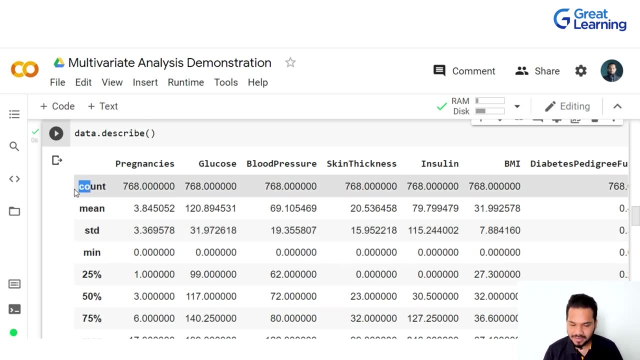 people who are, uh, you know, going on to giving me some data points out there. what are some of the things that I can tell as of now with respect to a statistical description? well, the first, uh, the row here it says count, count is basically telling me how many entries there are with respect to that. 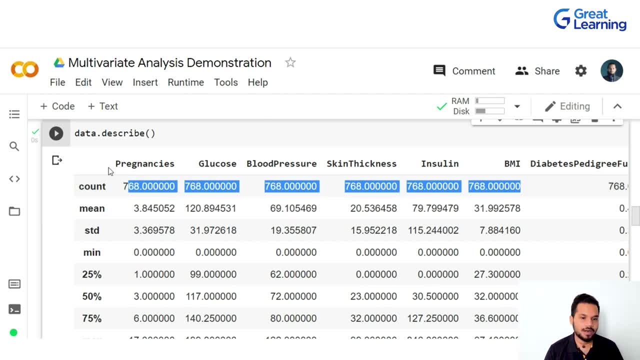 column. as you can see, it's 768 everywhere, so we don't have any empty uh columns or rows out here and it is giving me the mean of it. mean is basically the average right now in the entire 768 people. you can see that the body mass index average is actually 32, which means that overall, 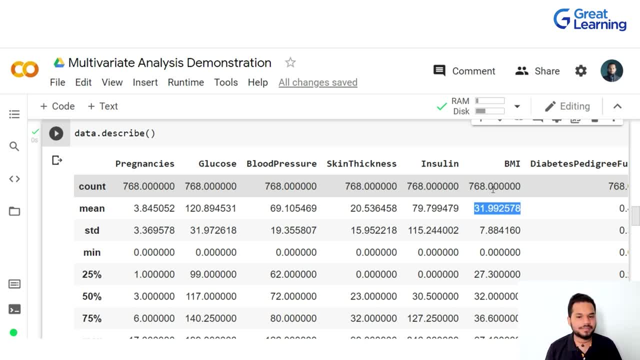 there are, if you consider this, uh, the data set in general. this is a hypothetical data set. the body mass index is slightly higher than what we would prefer, which is around 25, 26, 27, right, you can take a look at all that. you can take a look at the standard deviation. you can find the minimum values. 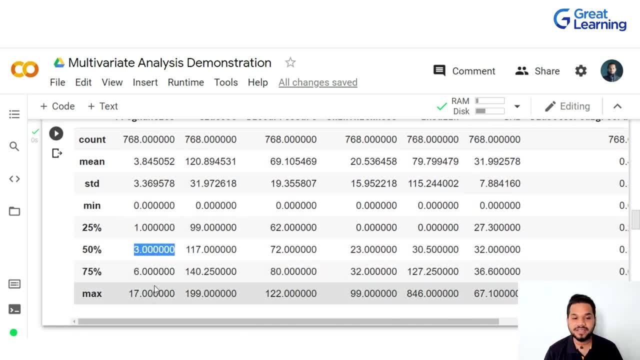 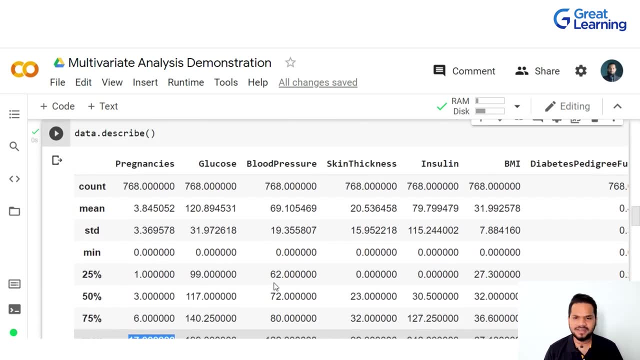 you can find out what is the value at the 25th percentile, 25th quartile, 75th quartile and eventually, even the maximum value. uh as well, right? so there are various things that you can figure out from this looking at it, as soon as you take a look at it. 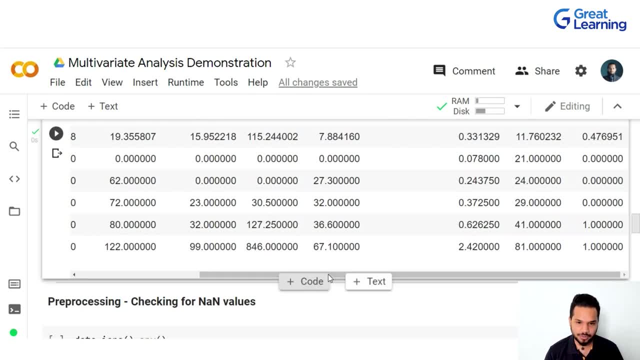 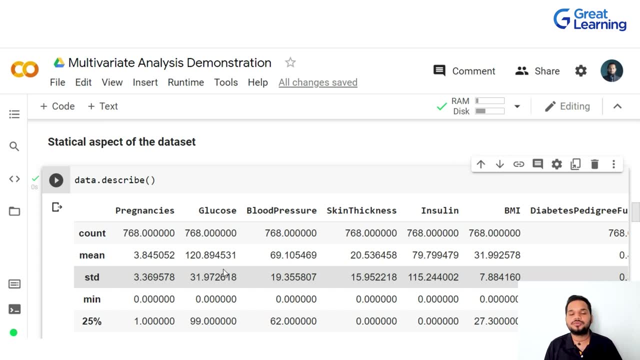 you'll be like, oh okay, so this is what is happening, uh, with respect to all of these, uh, individual entries. right, this is uh taking your entire data center instead of walking you through each of those 768 entries. this is me giving you a statistical aspect of it. say, hey, look at this with respect to 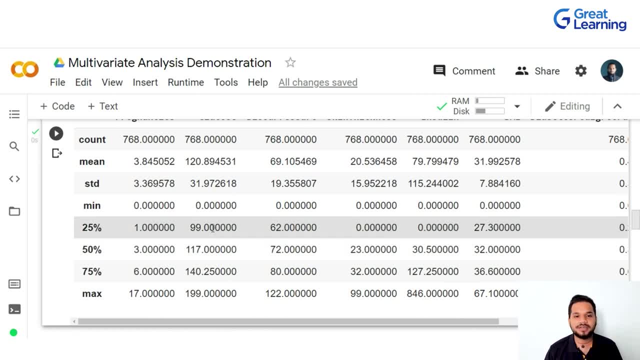 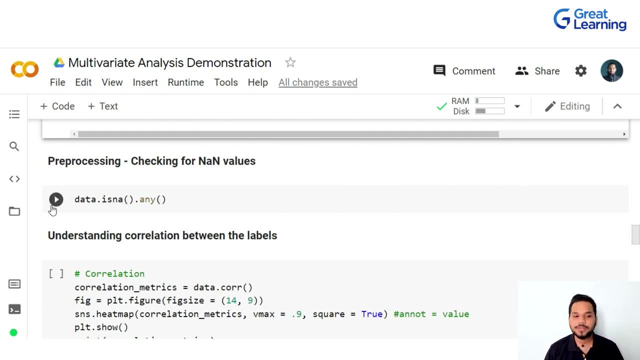 data that we use with respect to data not described done. we just used it and we realized that we can find out so many things about our data set right now. the next thing is the part where we'll actually be performing some pre-processing with the data now. thankfully, in my case, I do not need to perform. 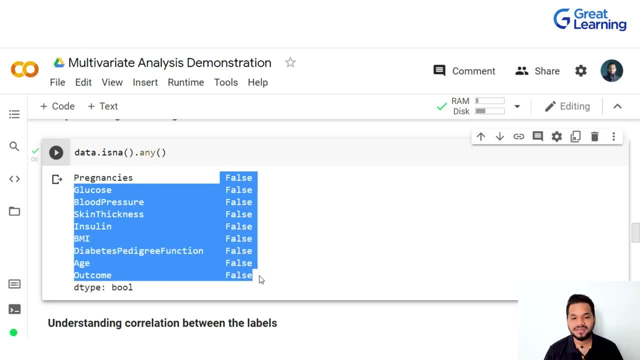 any sort of uh pre-processing here, because all of these values, wherever it says false, it means that there's only numerical values that are found. is any is basically telling? is it not a number? is it anything apart from a number? so wherever it says false, it means it's a number correct. now again. 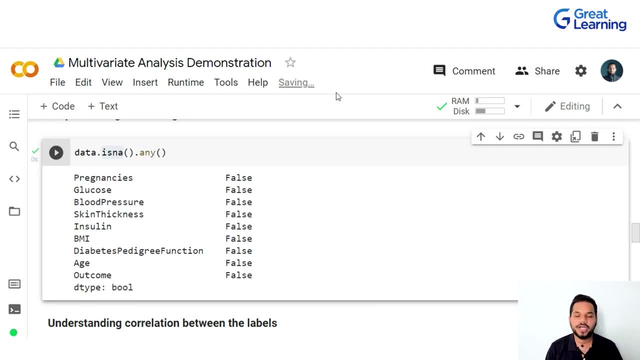 I told you right when. so when I ask someone: hey, what is your body mass index? please import it into this column. they might have written O, positive blood group right. of course they don't do it on purpose, but it is done by mistake and if it says true here, in many of the point of cases it means 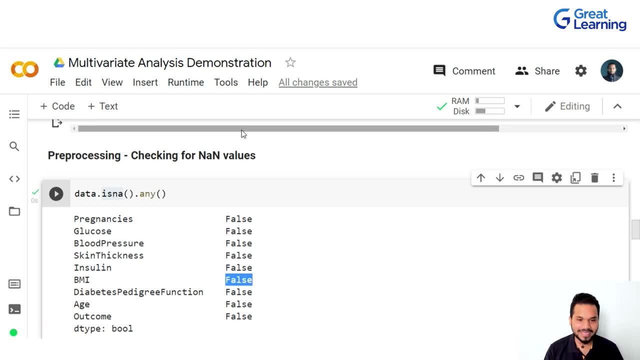 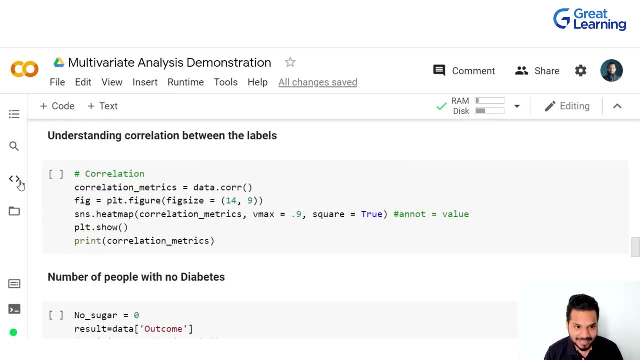 that that there is a wrong entry there, that you have to go and fix it up. now. in my cases, I told you: this data set, this hypothetical data set, is already cleared. I don't have to perform any sort of pre-processing on it. the next thing that I can jump directly is to understand this concept called. 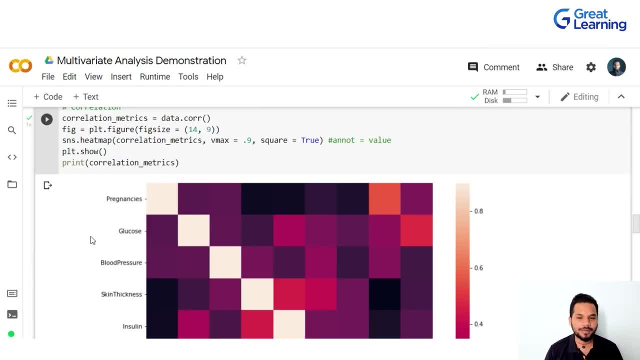 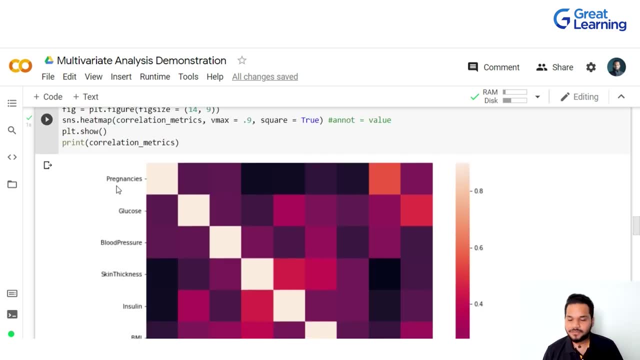 correlation. correlation is a beautiful concept, especially for multivariate analysis, because here it will tell you how much of dependency exists between two variables. right, first of all, take a look at the heat map on the right. if it is, of course, it's positive correlation. there's negative correlation. all of that to 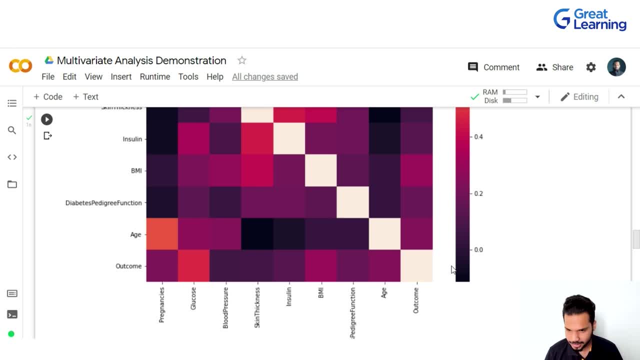 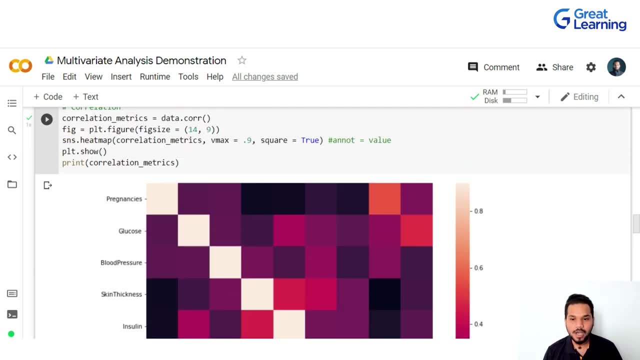 simplify it for your case, where you're just going to be talking about positive correlation here. now, whenever there is this chart that starts from 0.0 all the way to one, you can see the color lightens. when the color lightens in the legend, it's basically telling you that whatever if it. 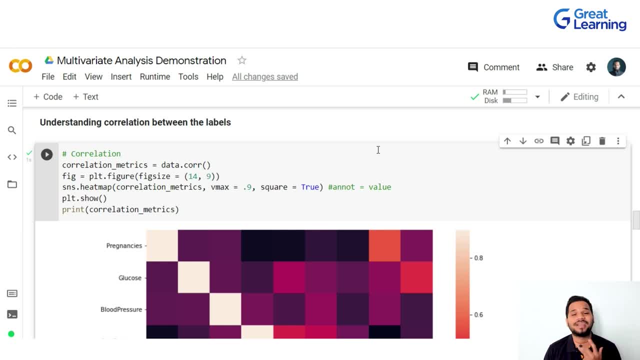 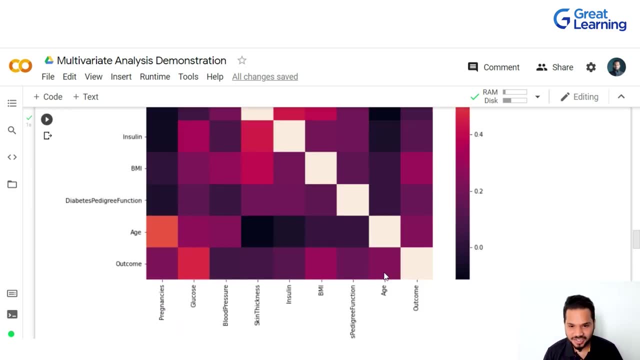 is that color, that is the amount of positive dependency, the correlation that exists between, uh, these two variables right, for example, pregnancies and age. right age is your pregnancy is here, so this is the box that we're talking about. you can see that this is light in color compared to all the. 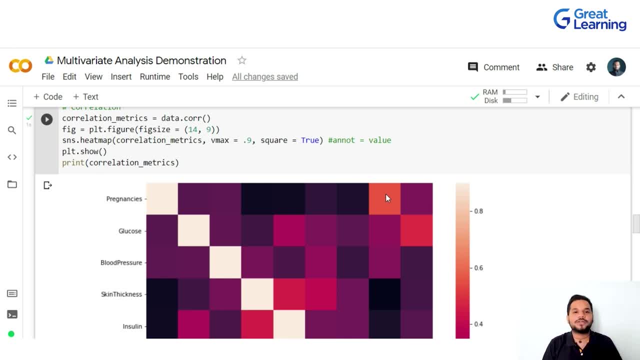 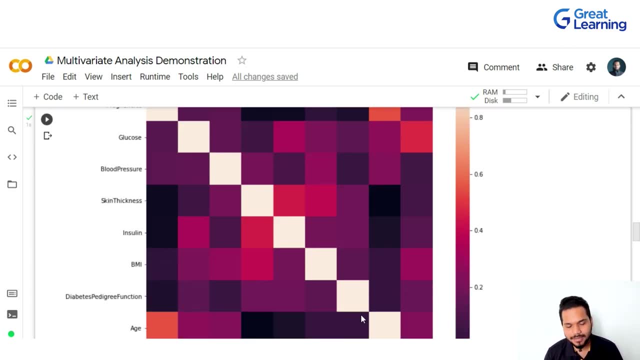 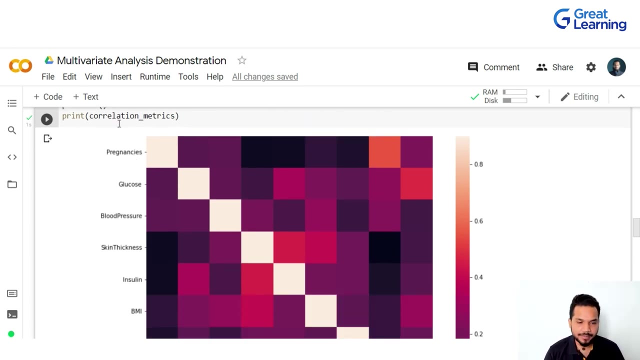 other boxes, right. so pregnancy and age has a good amount of correlation there and wherein the uh? you know you could figure it out just by looking at your data. now you might be looking at the diagonal. it's exactly equal. yes, it is exactly equal. I'll tell you why it is white, because, if I have to, 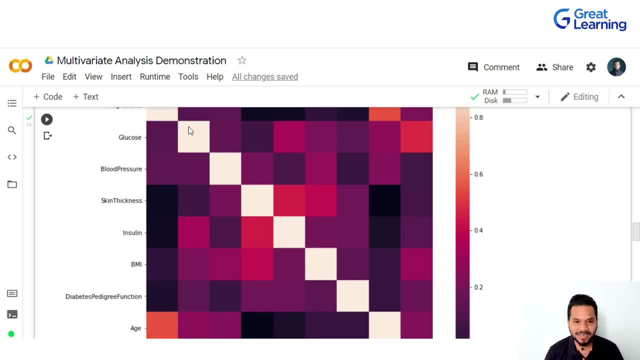 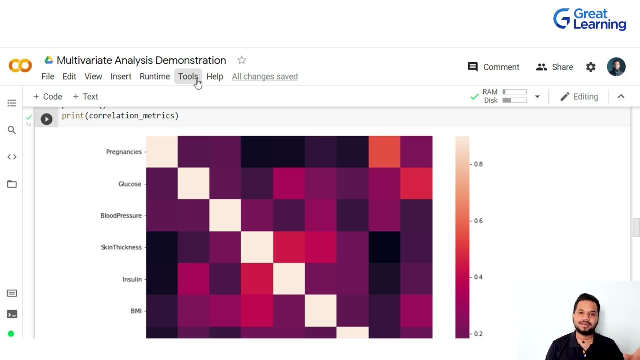 compare the value of glucose. now, this is white. what are we comparing it with? let me scroll down. I'm comparing it with glucose itself: glucose compared to glucose for any person, if it is like 300 versus 300, isn't it exactly the same thing? yes, similarly for blood pressure. skin thickness. 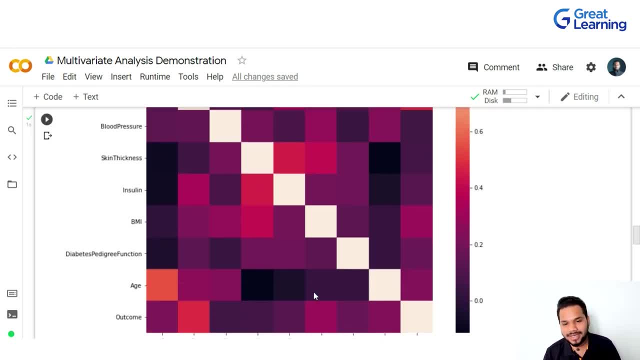 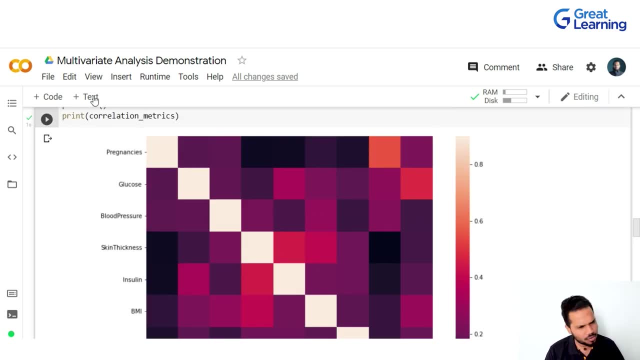 insulin, BMI, all of these different parameters- you have to take a look at it- wherein each and every one of those, when you compare it with the exact same thing, it's always going to be 100, equal right. so all the diagonal elements will always be- uh, you know, uh- be white. 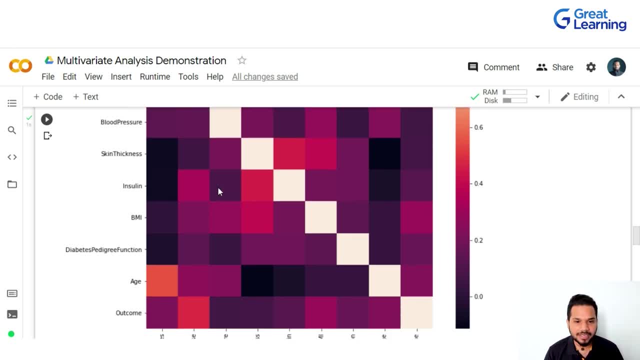 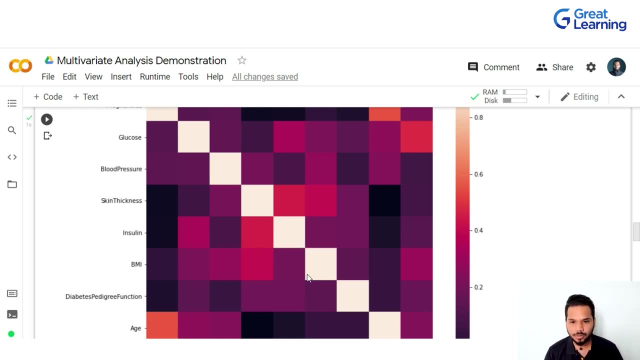 in color. right, so you can. you can analyze various points here. for example, take a look at insulin and skin thickness. insulin has some sort of relationship with skin thickness because this is a lighter color compared to all the shades around it. right, so like this, you can actually sit for a couple of minutes. 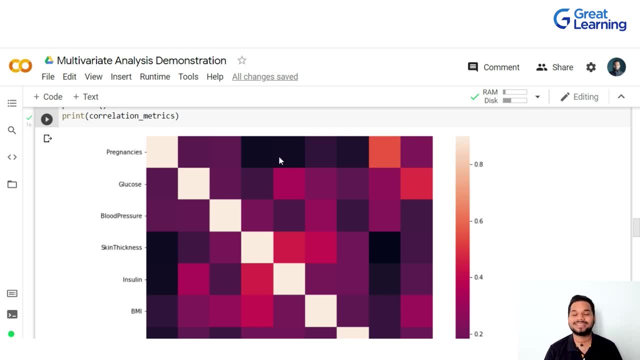 try to analyze and try to write down what are some of these uh correlations which are, which will be very important for you to later not only understand. these are the variables that have the outcome with respect to correlation. you can say: these are the variables that have so and so outcome. right, you can give attach a numerical metric to it. 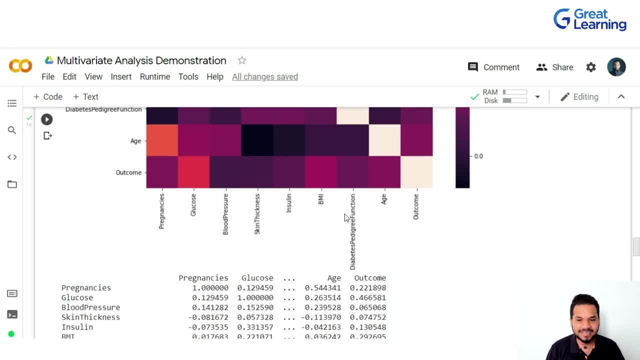 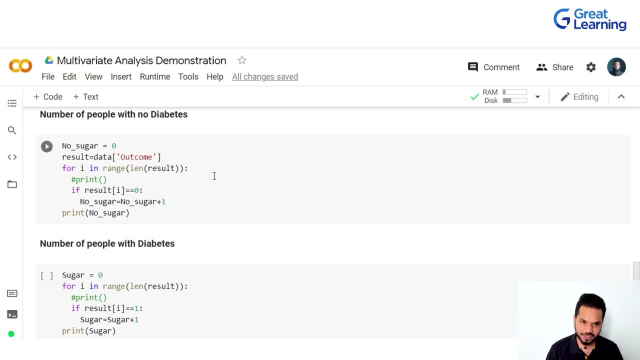 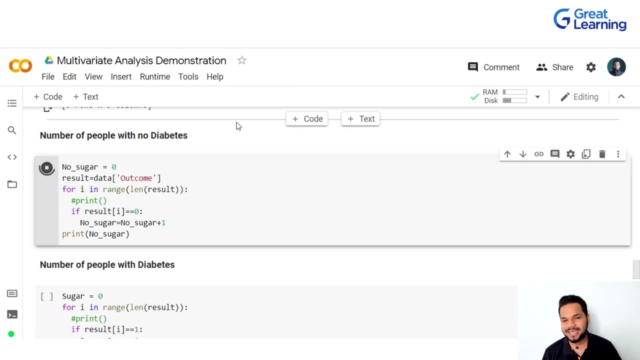 to say: hey, uh, you know, pregnancies are 80 related to, or age factors or something like that. you can always go on to perform. uh, all of that with respect to a simple correlation Matrix. now we know that we have 768 people. how many people, how many people do we have who have no diabetes right as soon as a? 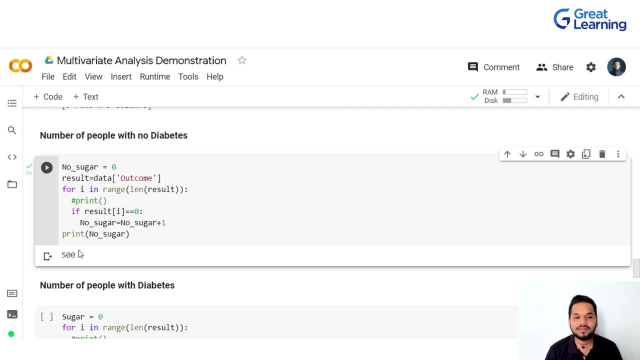 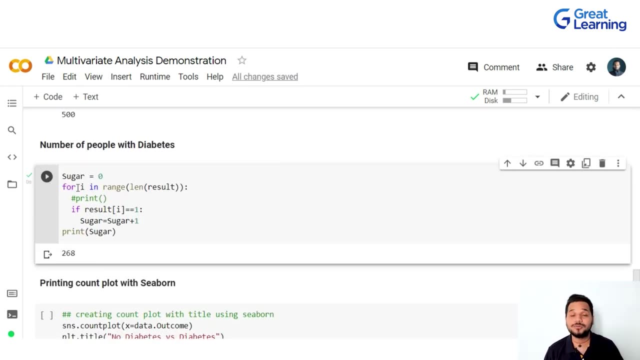 few lines of code, three or four lines of very simple logic, will tell me that there are 500 people who don't have diabetes. another piece of code tells me that there are. of course, if there are 500 people who don't have diabetes, it is 268 people who have diabetes. now you might be saying: 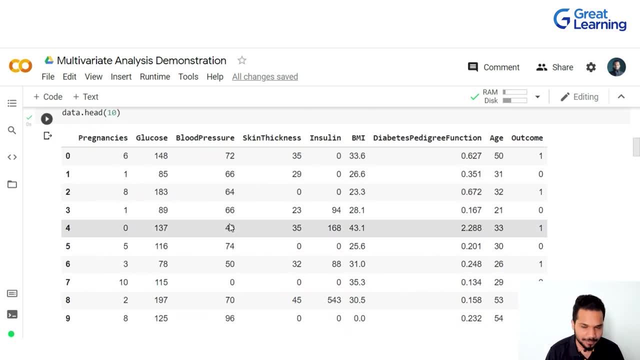 hey, wait a minute. I didn't understand. how did you figure it out? let me scroll up to the data set and you can see this last column: one and zero. one and zero, right. so all I have to do is I have to filter everything here. if I just have to pick up everything, that is one and count how many are there? 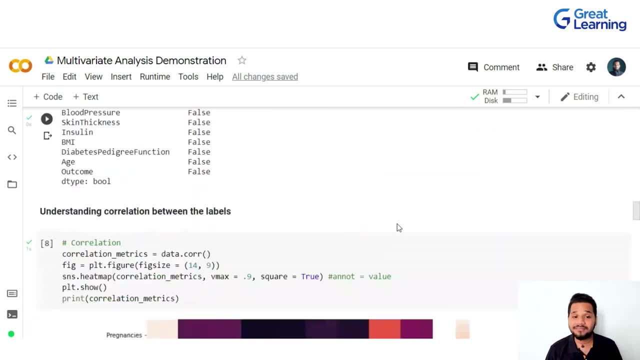 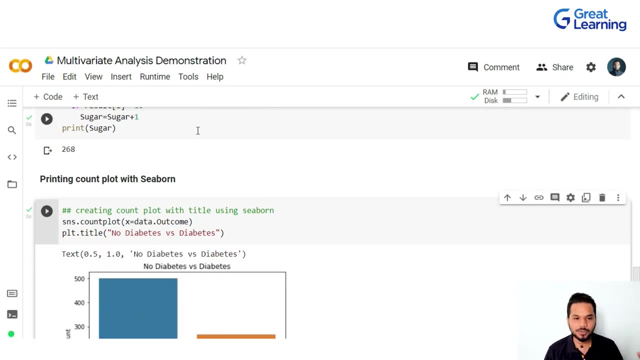 count how many are there. that will give me the total number of people who have diabetes and who do not have diabetes. right, that's all I did, but if you still want a simpler explanation, as always with the help of data visualization, you can take a look at it. if the outcome is zero, it means the 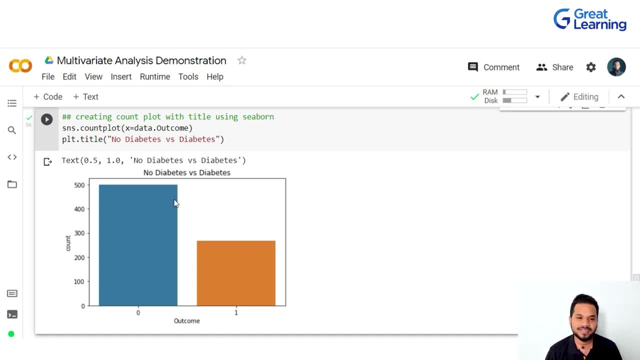 person does not have diabetes. if the outcome is one, it means the person has diabetes. now you can see that it it is a sharp market. 500 means 500 people don't have diabetes and here are somewhere around 268 people. roughly around 268 to 70 people have diabetes right now. you can see that it it is. 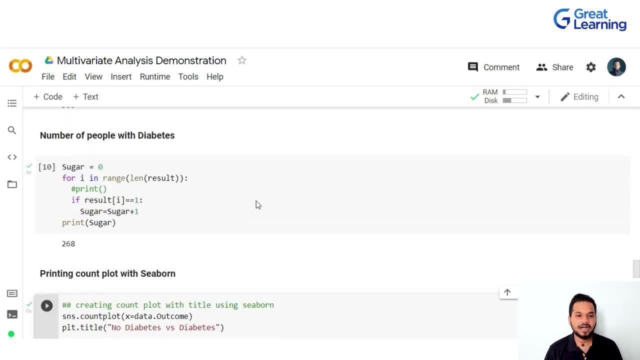 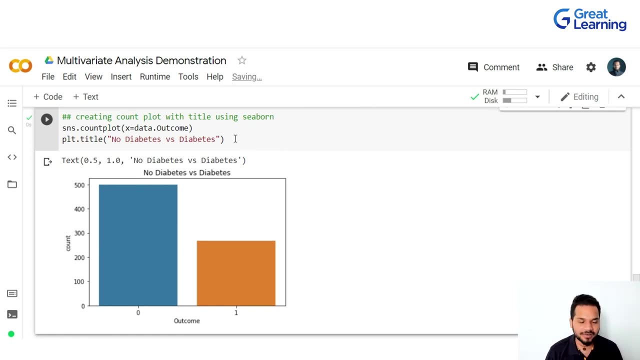 you know, you can just look at this graph and within two seconds you can figure it out. uh, if you're a person who says, oh, I don't really like to like write all of this code, just to find that out two seconds, create a- uh, you know, try to create a plot and you will have all the details in front. 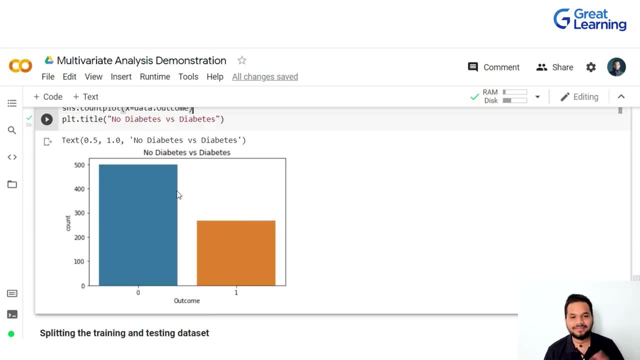 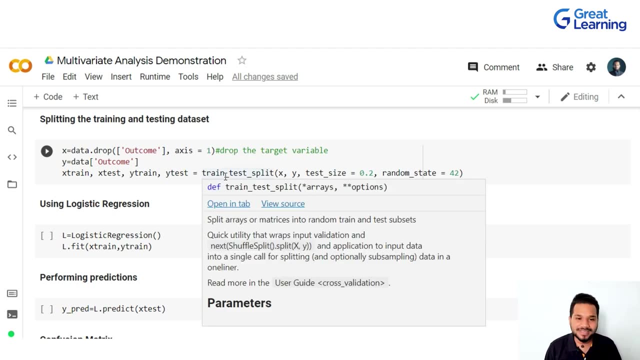 of you right. the next couple of steps are pretty simple now. multivariate analysis is where now. now is where machine learning takes over a bit. the next thing that we need to do is we need to break the data apart into two pieces. one is the training data set and the other one is the testing data set. 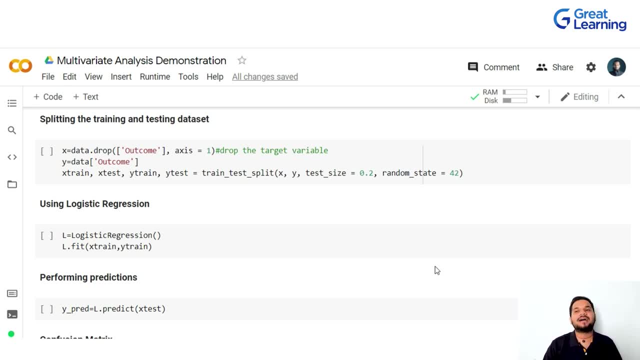 why is this done? well, this is: we want to make sure that you know we have brand new data that our machine learning algorithm can test later on. it's just like your college examinations: you read using your textbooks, you close your textbooks and eventually go write your examination from your memory. why is that done? 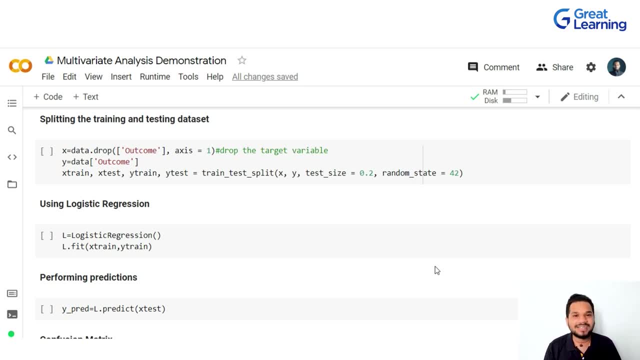 that's done, to see how we have learned, what it is that you have exactly learned from those books. we want you to reproduce your learning right. similarly, if we divide stuff out into two pieces and if we hide one piece for a later- uh verification stage, we can understand and we know that it has learned. 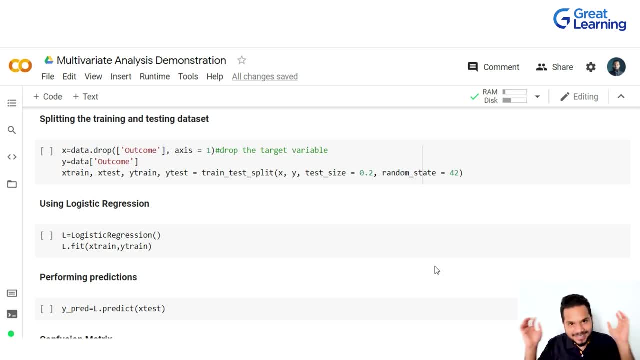 it better, right? because if I give it the training data right now and later send the same training data again, it will give me 100 result. it will say, hey, everything is correct. that's not what we want, right? it's. it's like having your textbook next to your examination. we don't want that. so basically what we're trying: 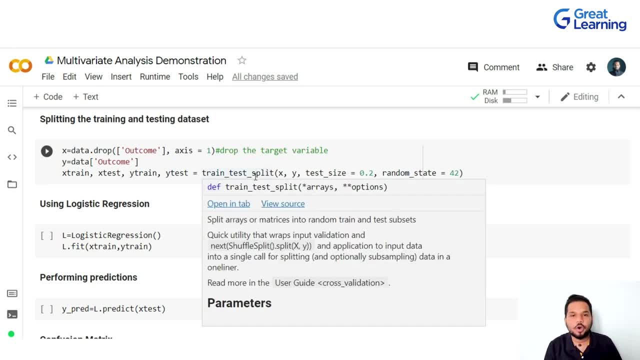 to do is when we are providing the data to our machine learning algorithm. that last column with said outcome, where it had the details of if a person has diabetes or not, we're going to drop it, we're going to remove it straight away and we're going to break the data into two pieces. 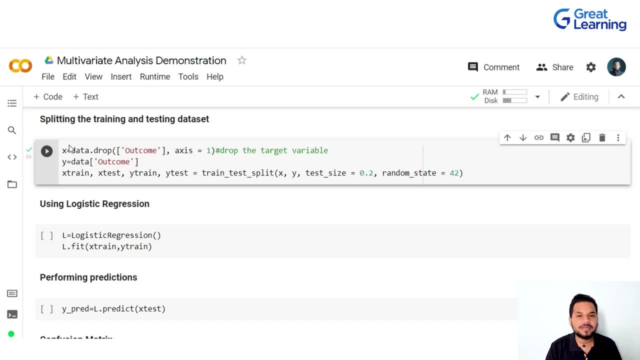 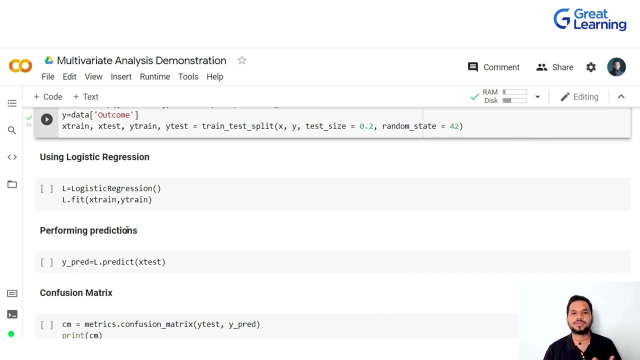 one, one chunk. one basket consists of eight pieces, and then we're going to divide it into two pieces, so 80 of data, while the other basket consists of 20 of data. now, for all the people who are not used to machine learning, if you're a person who's thinking, oh, I'm going to require hundreds of 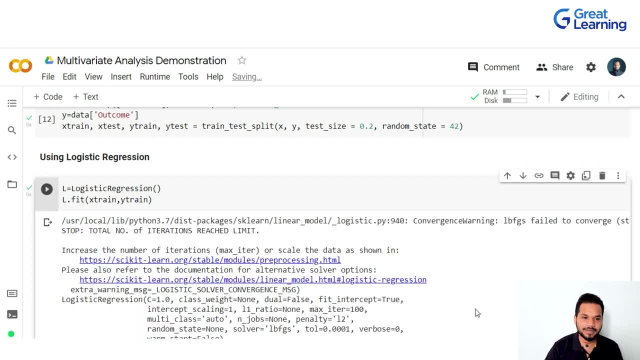 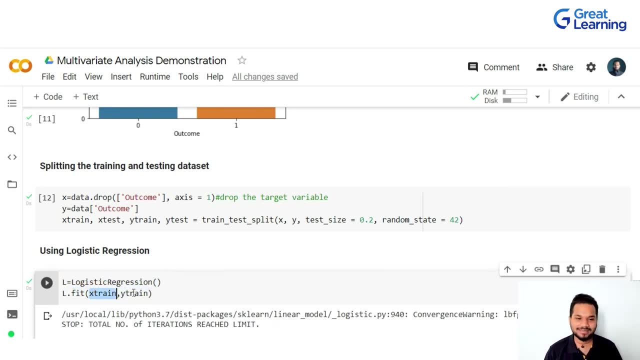 lines to perform machine learning. not really. as soon as I click this uh particular code snippet, here are these two lines that you see. uh l equal to logistic regression and model fitting is a place where we actually provided it with respect to the training data, and as soon as this is done, 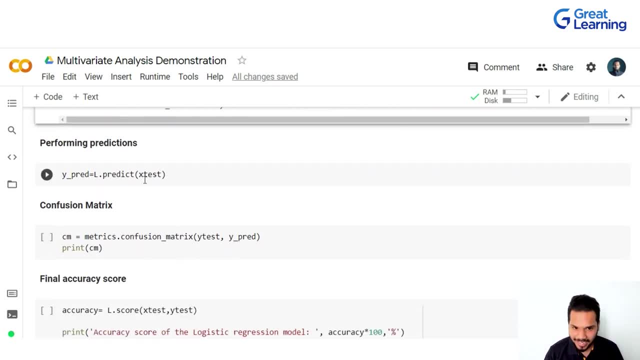 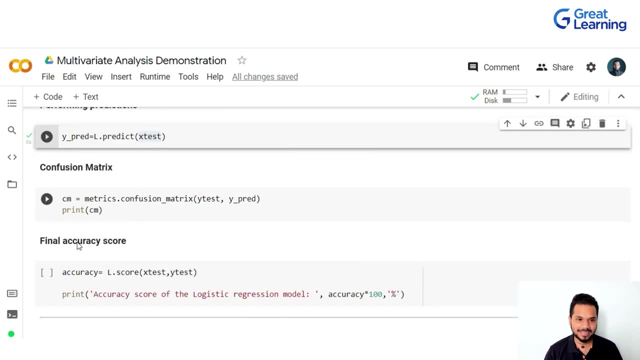 the model has actually finished learning everything. the next thing is where I give it that test, where I say: here is new data, tell me if you can predict this correctly. and with again one line of code, that is done, and after that you have one more. all of these are basically statistical concepts. 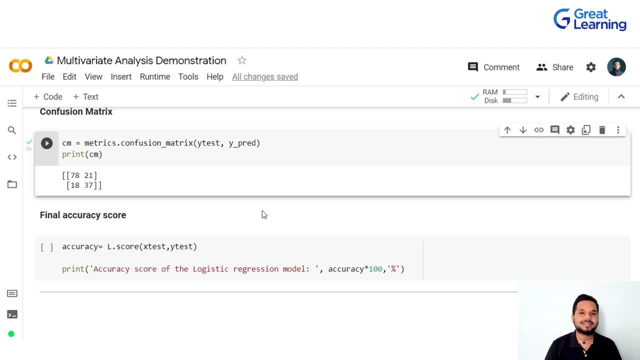 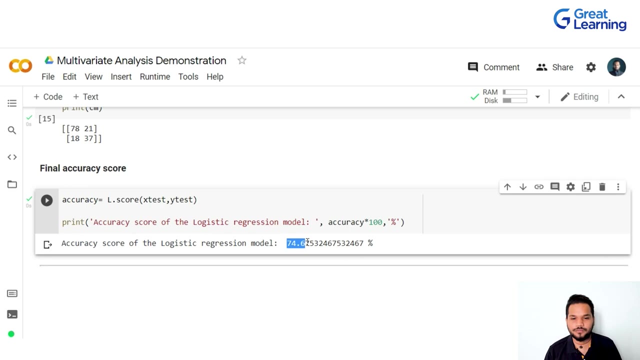 so it's the measures of accuracy. here there are concepts such as true positives, false positive, true negative, false negative. those will actually be used to assess and gauge the performance of your machine learning algorithm. but for simplicity's sake, let's have an accuracy score. it says the accuracy score is seventy four point six, seven percent. all that it is trying to tell us is: 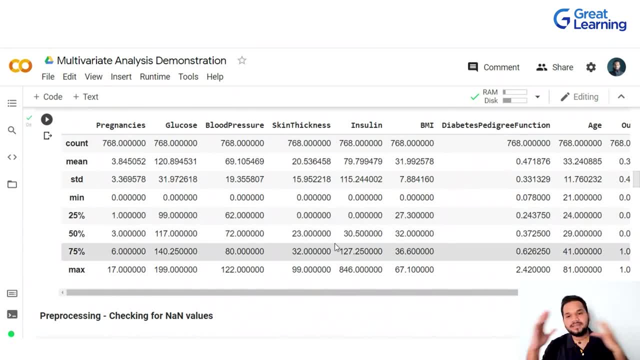 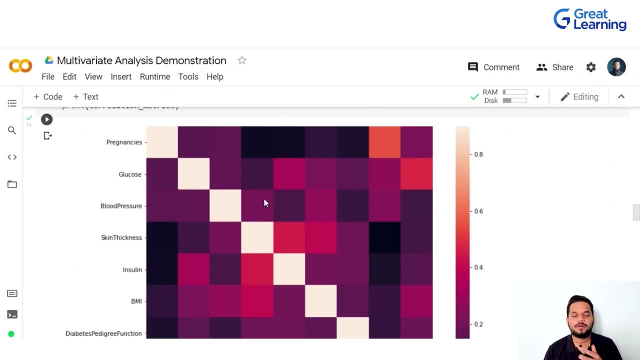 this machine learning algorithm could figure out what are the various uh factors. that's going to lead to analysis, that's going to lead to diabetes, and we made sure to take a look at it manually with respect to performing MVA over using correlation uh. once we did that, we figured out how many people 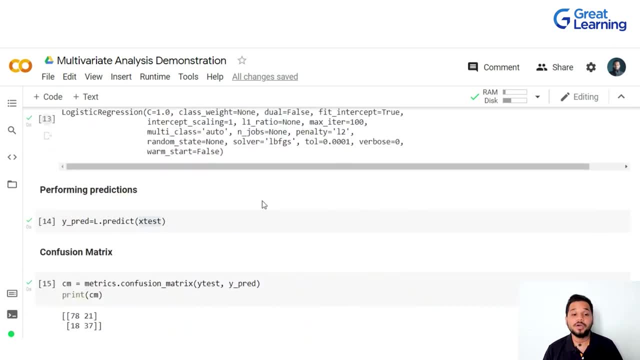 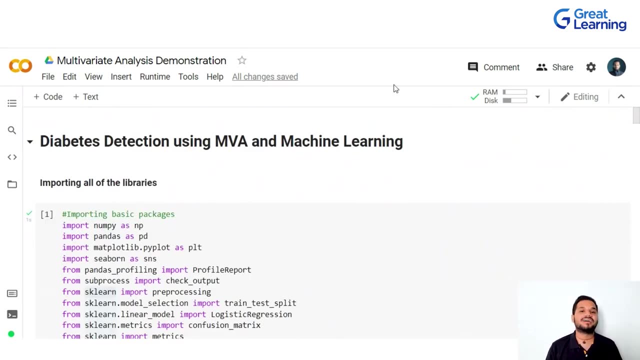 have diabetes. how many people don't have diabetes? we printed a small graph, we used logistic regression and at the end we printed out an accuracy score to say, hey, by not only just performing our feed it into a machine learning algorithm and get the machine learning algorithm to predict if. 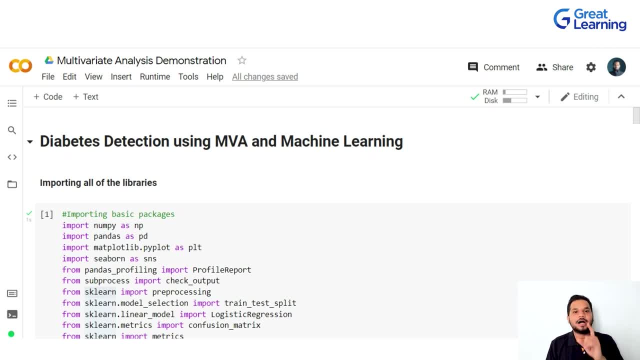 something if it can find out if the patient has diabetes or not. how fantastic is this? right? we started out by thinking, hey, this demo will only be talking about multivariate analysis. we also made sure to complete, have a bigger view at the picture, to tell you- not to tell you exactly, not just how. 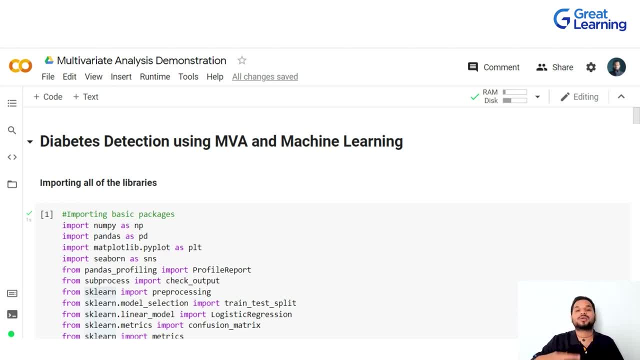 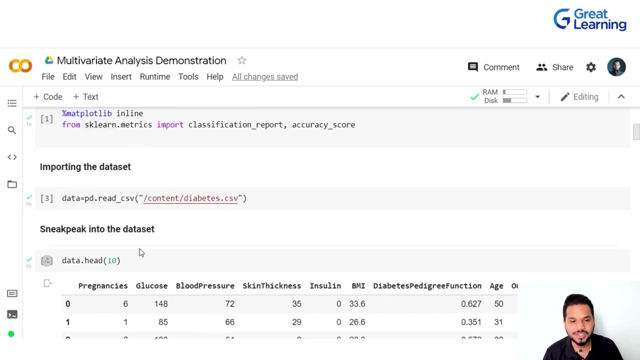 uh, multivariate analysis works, but again, whenever you think about where it is used, this is where it is commonly used- it is attached with either machine learning or machine learning to drive insights based on those results. it's very important for you to understand that and, as I just told you right, the goal here for you to is actually to understand the structure. 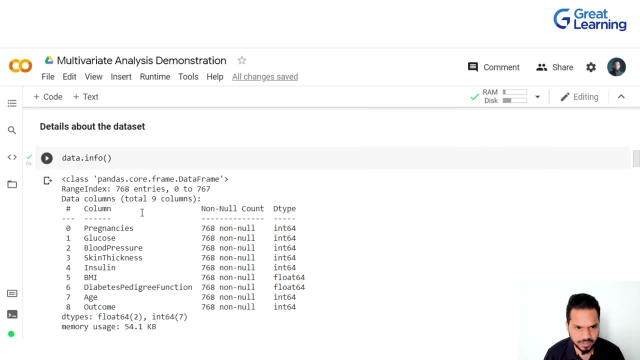 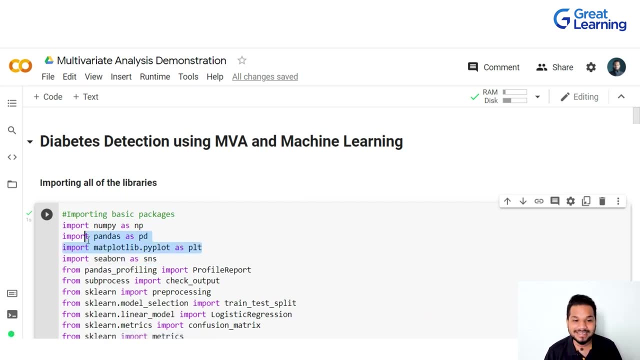 to understand how we try to attack this particular problem and solve it. and, of course, there might be some of you who are watching this course right now who might be saying: hey, I don't know why you've written this exact line like this. yes, you're going to require a bit of introduction to python to 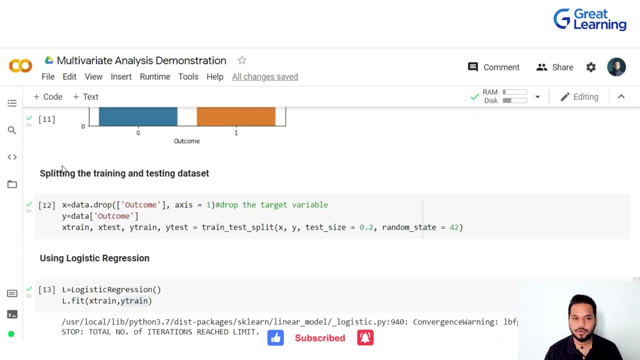 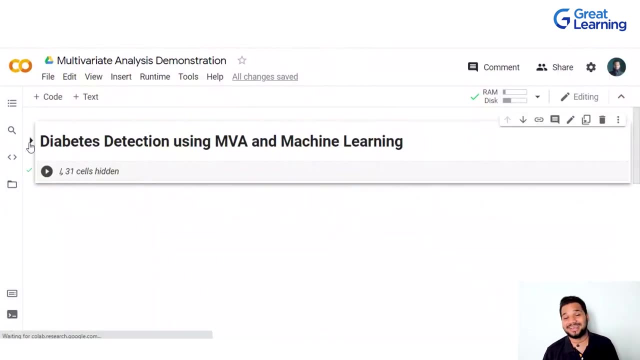 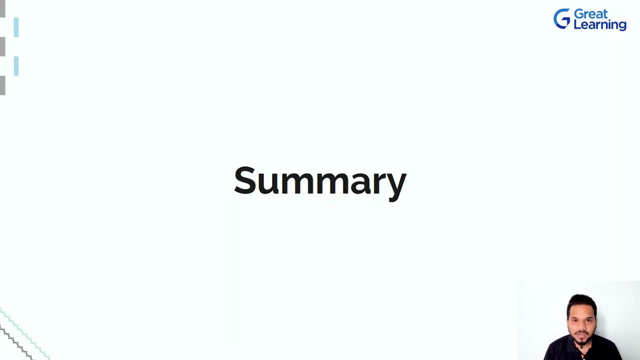 understand how python syntax is written. uh, to actually go on to figure all of this out in detail, but I know so that's not the goal here. the goal here was to show you a multivariate analysis and also give you an extended view about using machine learning there as well. well guys, with this we have come to the end of the. 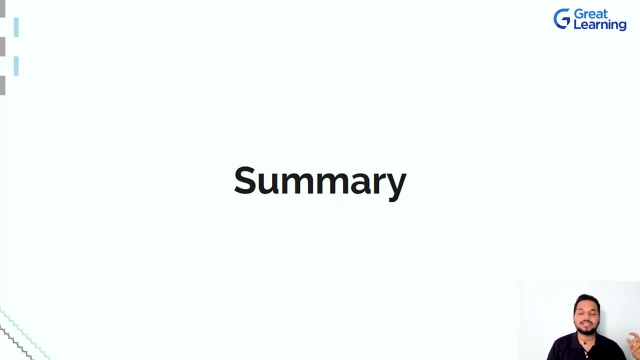 course. thank you so much for watching. we started this one out by taking a look at understanding what data analysis basically is. once we figured out what data analysis is, we took a look at the various types of data analysis we could perform. once we understood the various types of analysis. 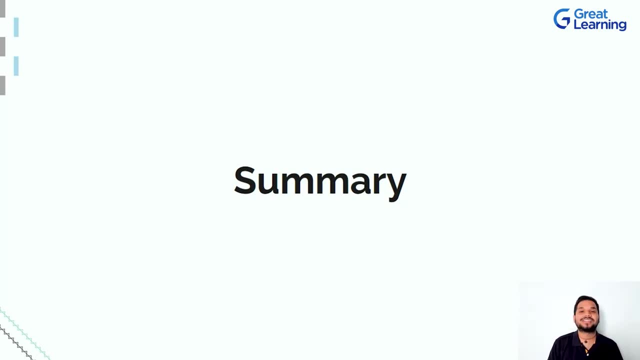 again with very good examples. we homed in on multivariate analysis. we started understanding what is multivariate analysis, where it is used, what are some of its popular applications, what are its very good techniques that are used everywhere around us, what are the advantages of it. and we also made sure to take a look at practically implementing.